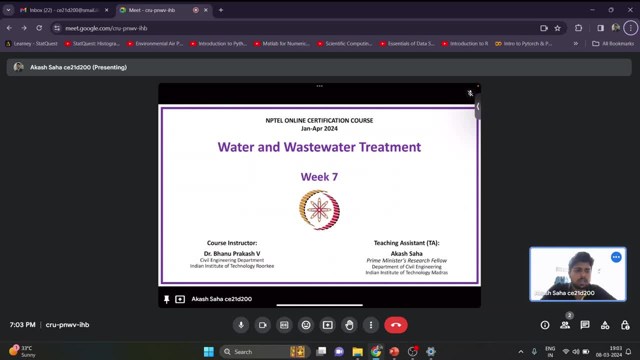 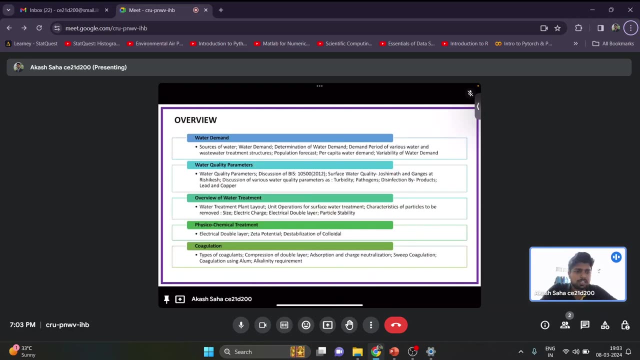 My name is Akash Sahar and I am a PMRF scholar at the Department of Civil Engineering at IIT Madras, where I am pursuing my PhD in Environmental Engineering. So we will quickly go through the contents of week 7.. In week 7 we started with the water treatment, where we first 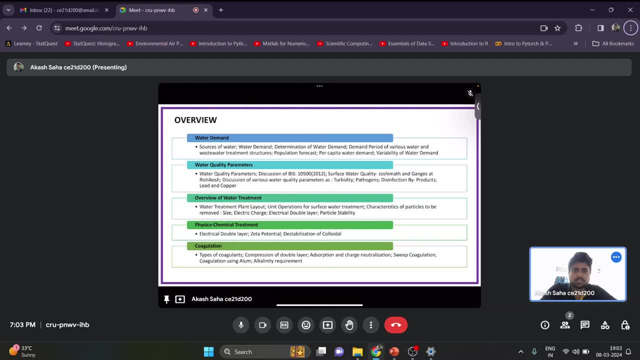 saw about the water demand and what are the various demand periods of various water and wastewater structures, the population forecasting, the per capita water demand and the variability in the water demand. And then we moved on to the water quality parameters, where we discussed about the BIS10500. 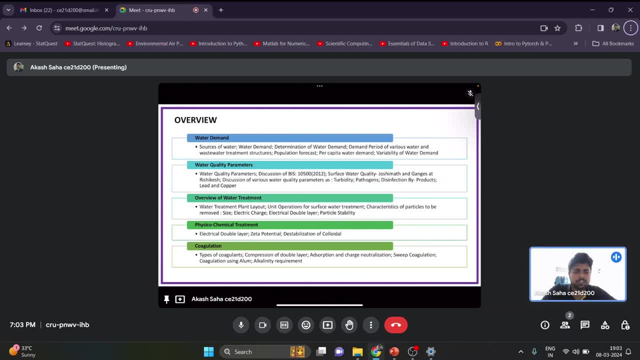 which is the standard code, and many surface quality water quality parameters like the turbidity, pathogens, disinfection by-products, lead, copper, etc. And we also saw the case study of Joshimut and Ganges at this research And then we moved towards the overview of. 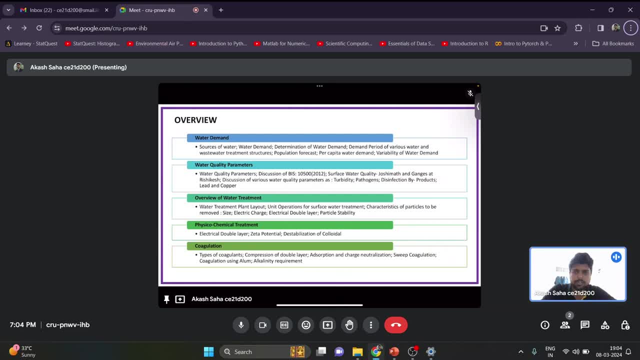 the water treatment, where we saw the layout of the water treatment and the per capita water quality parameters, The layout of the water treatment plant, the various unique operations for the surface water treatment, the characteristics of the particles that have to be removed, their electric 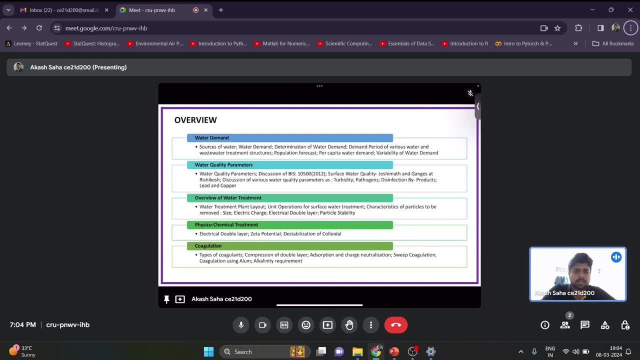 charge, the concept of electrical double layer and the particle stability. And, moving on to the physicochemical treatment, we learned about the Zeta potential and the destabilization of the colloidal particles, And then we moved on to discussing about the coagulation, Like 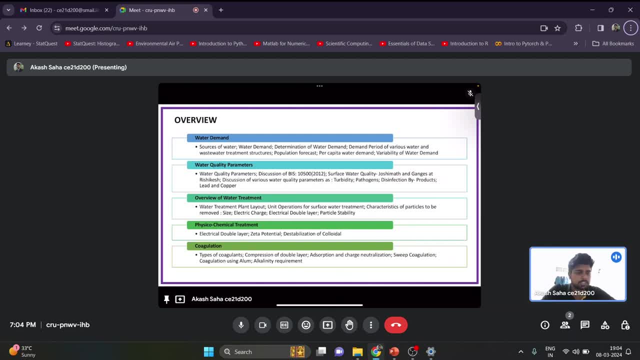 what are the different types of coagulants, what is the compression of the double layer, absorption and charge neutralization, the sweep coagulation and how we can do coagulation with the help of alum, and what is the alkalinity requirement. So this was the brief overview. 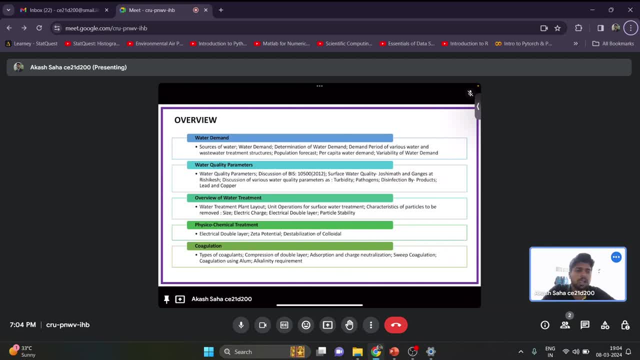 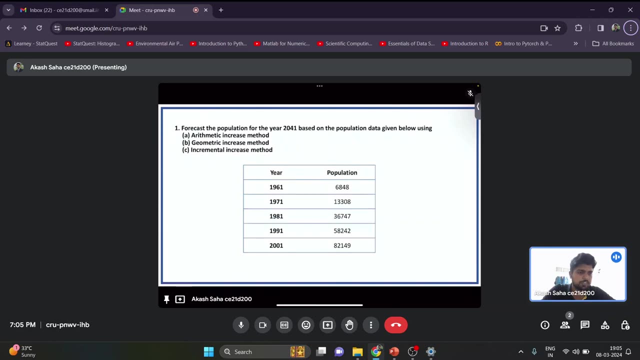 of the concepts which we saw in week 7.. And now we will be solving some of the questions, both subjective and objective, So we will go through the question one by one. Okay, So this is the first question, which is related to the population forecast. So 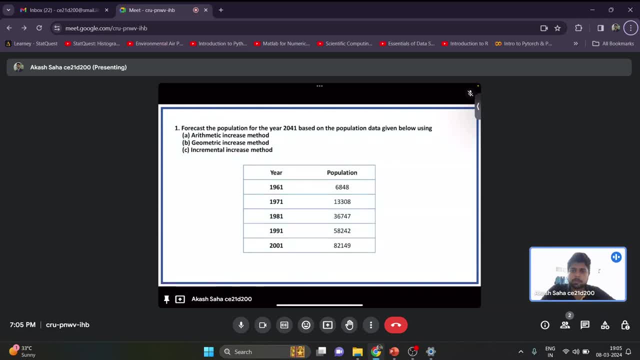 it says that focus the population for the year 2041, based on the population data given below, using arithmetic increase method, the geometric increase method, the incremental increase method. So we have been given the populations corresponding to five different years, starting from 1961 to 2001.. So the populations are given for a period. 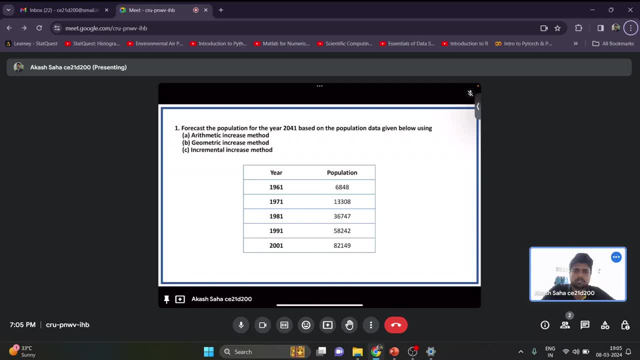 of 10 years, So per decade, what is the population it has been given. So you have to forecast the population for the year 2041 and we have to use all the three methods, starting from the arithmetic increase method, the geometric increase method and the incremental increase method. So I will 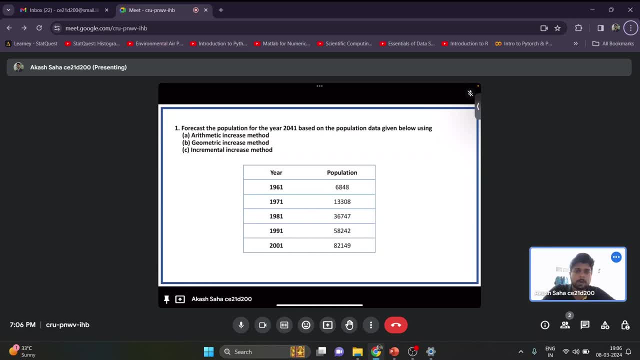 give you some time to note down the population and then we will see how to find out the population, How to forecast the population for the given period of time. Please note down the populations corresponding to each year, So starting from 1961 to 2001.. 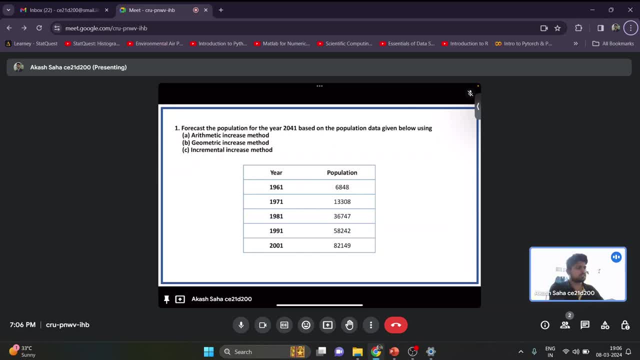 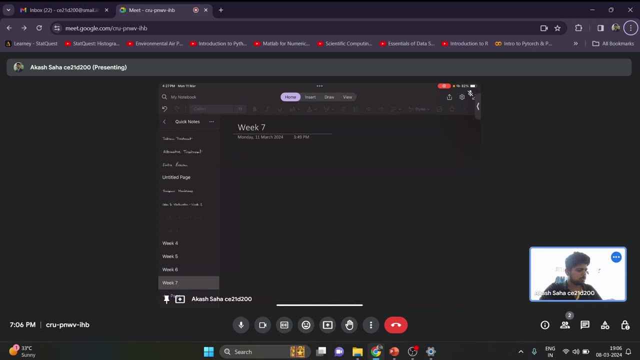 Okay, So we will see how to solve this problem. We will start with the arithmetic increase method. So we will start with the arithmetic increase method. So we will open my notepad. Okay, I hope that you can see the screen, Okay, So the first question. So we 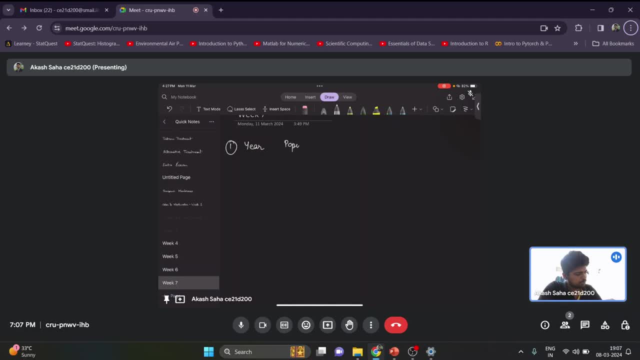 can say that we have the year and we have the corresponding population. Okay, So it is first is 1961, 1971, 1981, 1991 and 2001.. The corresponding population that is being given are, we can say, 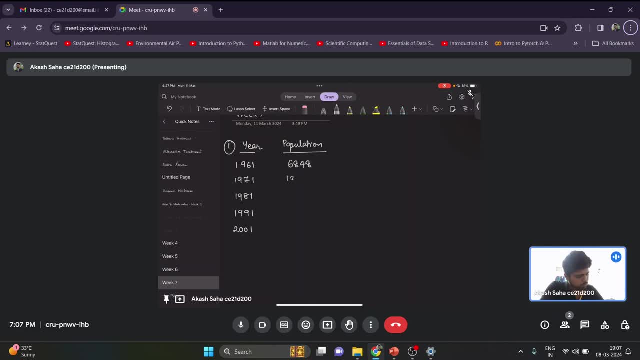 6, 8, 4, 8, 1, 3, 3, 0,, 8, 3,, 6,, 7,, 4, 7,, 5,, 8, 2,, 4, 2, and 8, 2, 1, 4, 9.. 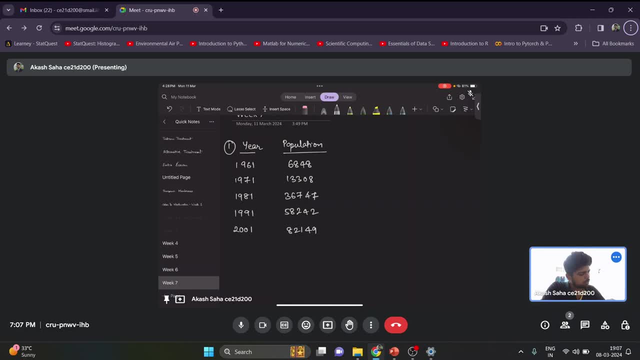 So these are the populations. So if we find out the change in the population, So first we have to find out the change in the population. So if we see the change in the population, So with respect to 1971, with respect to 1961, what is the change in 1971?? 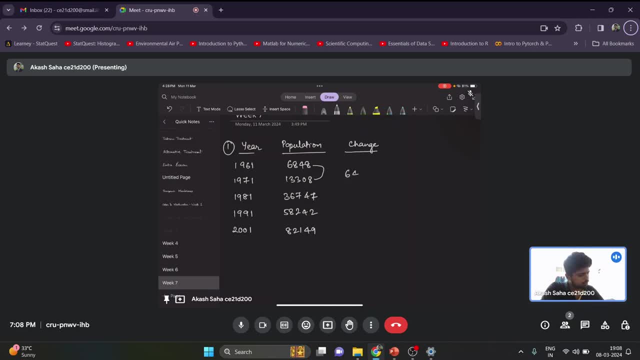 So if we subtract these two, we will get 6, 4, 6, 0.. Similarly, with respect to 1971 to 1981, we will get the change as 23,439.. So we have to just subtract the population. 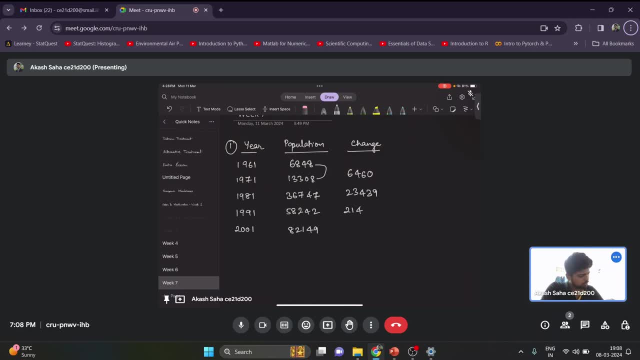 So in this way we will get the change. So I think these are the four changes we can find. So we have to just subtract these populations from the earlier population And then we will find out the total, The total. 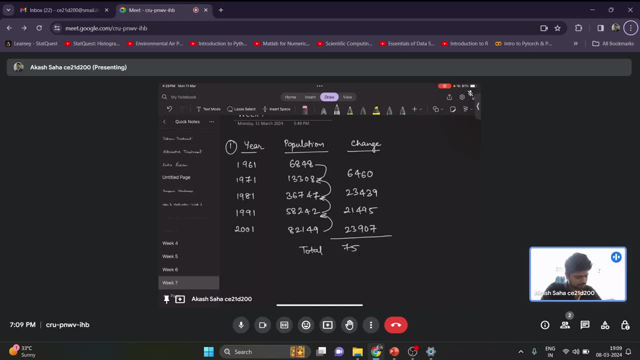 So if we add all the changes, we will get 75,301.. Okay, And also we have to find out the average. So the average of these population will be equal to 18,825.. So we got the total and the average. 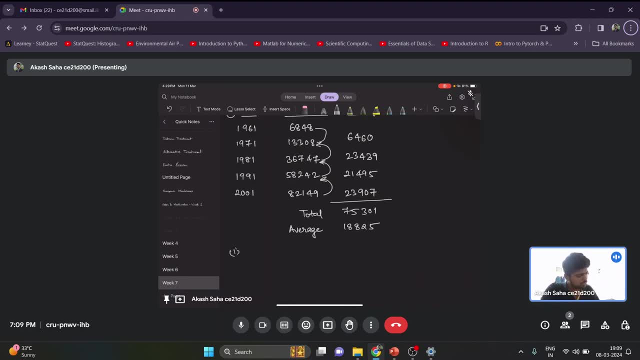 So now we have to. now, the first one is the arithmetic increase method. So at 2041.. So if we see the number of decades from 2001 to 2041, it is 4 decades, So 4 decades. 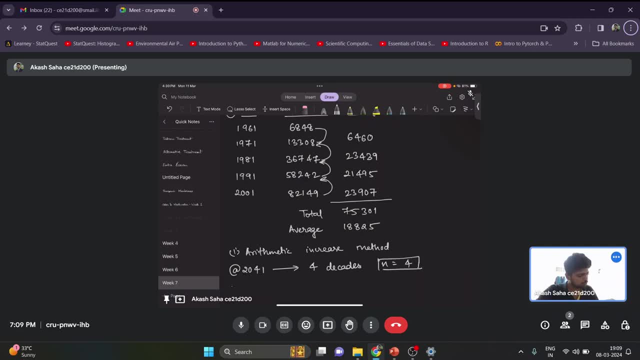 So our n will be equal to 4.. So the population at 2041 will be: So what is the known population in 2001? It is 82,149.. So 4.. So 4 plus the number of decades, that is n, that is 4 into the average increase in the population, which is 18,825. 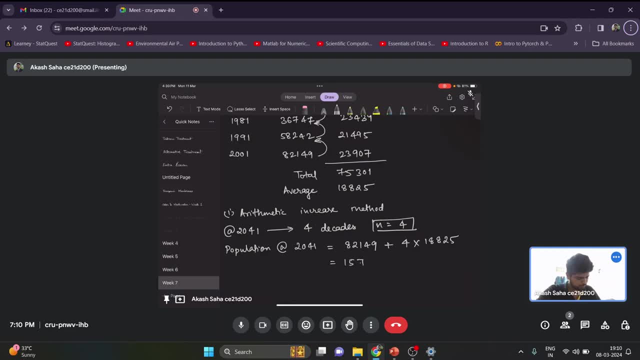 So if we calculate that, we will get the answer as 157,449.. So this will be my population at 2041.. So I will quickly go through the method of arithmetic increase method. So what we did, we will find the change by subtracting the two populations back to back. 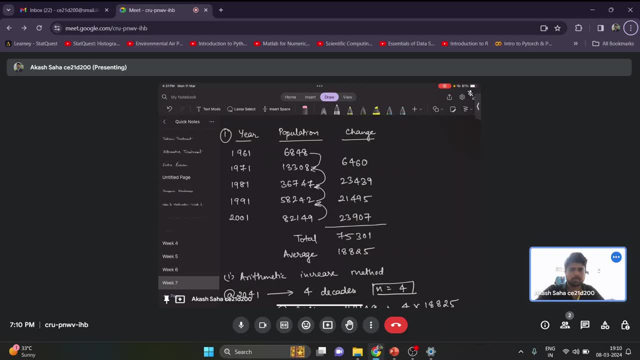 So we will subtract the population of 1971 from 1961. So like that we get the changes. Then we will calculate the total population and then the average population. So we will calculate the number of decades. that is 4, which will be my n. 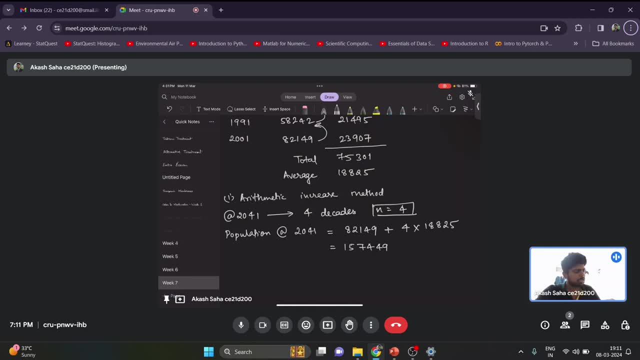 And the population in. So 1041, will be the last known population plus n into the average population change. So that will be the answer for the arithmetic increase method. Now we will have to find out the answer for geometric increase method. 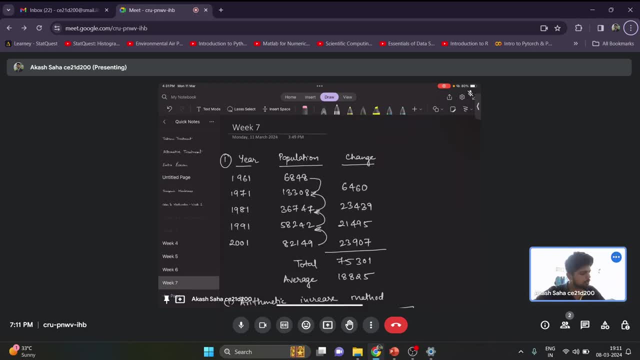 So for that what we will do, we will find out the percentage change, We will find out the percentages. So the first percentage change will be: suppose the change was 6460 and the population at 1961 was 6848.. 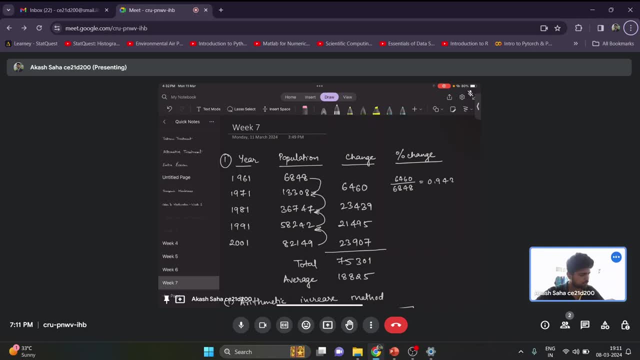 So my percentage change will be 0.943.. Okay, Similarly, for the next year, it will be 23439.. Okay, So we will add by 13304.. So my percentage change will be 1.765.. 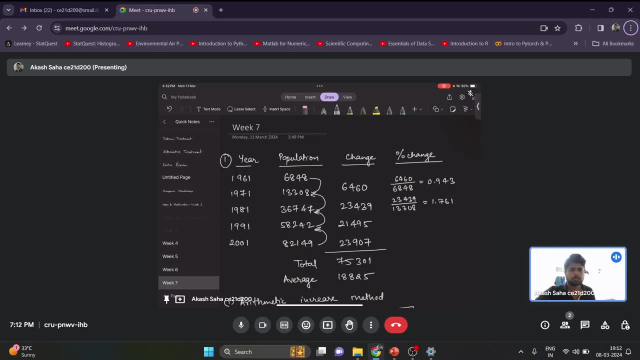 So, like that, I will find out the percentage change. So please calculate the other two percentage change by yourself. Try to do this. Okay, I hope you have been able to find out the percentage change. So for the other two years it will be 0.585.. 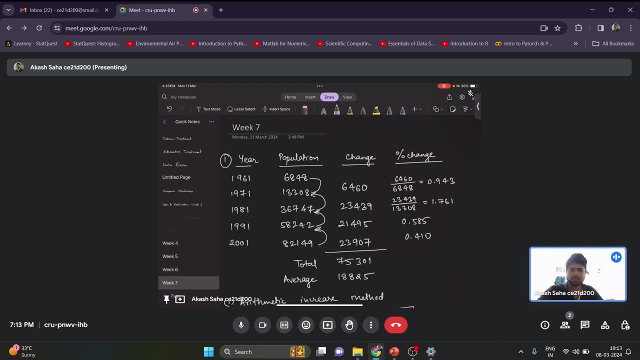 And then 0.410.. So we will find the percentage change. Now we have to find the geometric mean of these percentage changes. If we find the geometric mean, it will be equal to around 0.795.. Okay. 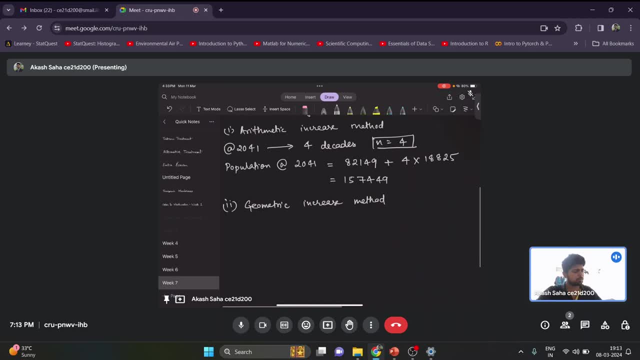 So this is my geometric mean, So we will see how to find out the population. So again, my n will be equal to 4.. Okay, So my n will be equal. So now the population at 2041, with the help of the geometric increase method, will be 8,. 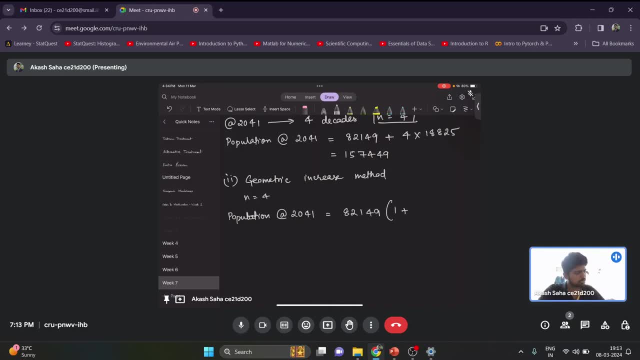 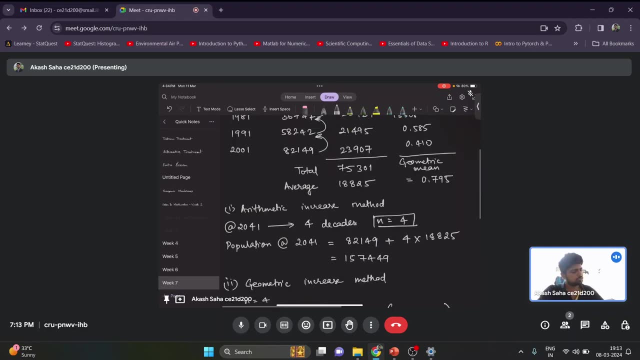 which is the last one's population, Then 1 plus r, So my rate will be 0.795, which we find out, which is the geometric mean. So this geometric mean So 1 plus 0.795.. 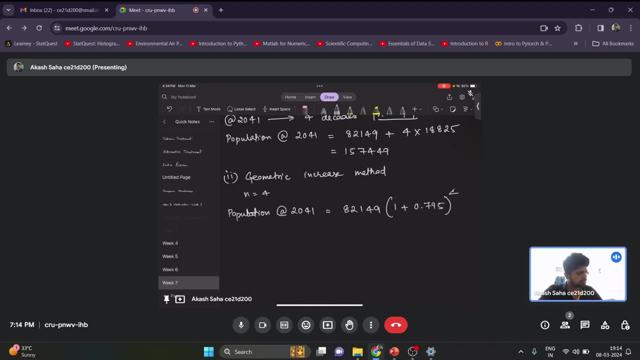 To the power, the number of decades. So that is my whole. So it looks like a compound interest formula. So where this is the p and this is r and this is n. So like that we can find out. 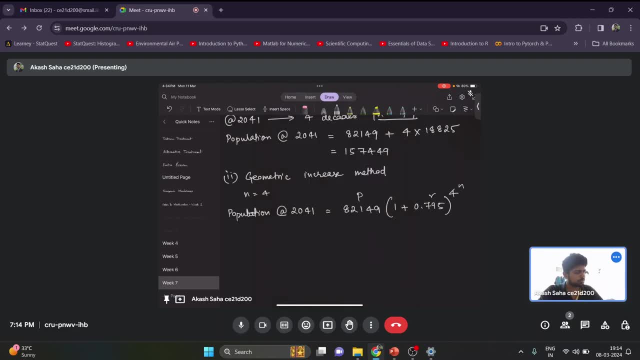 So this is nothing but the compound interest formula. So if we calculate this, we will get the answer as 8.. So 52331.. So we can see there is a drastic change in the population forecast in the case of arithmetic. 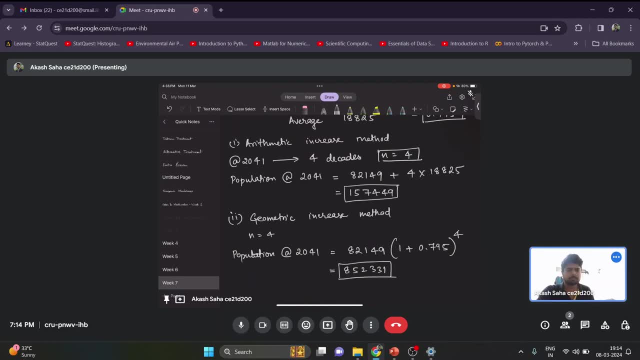 increase method. and in the case of geometric increase method, Okay, Because since we are assuming in the geometric increase method that the population will increase exponentially, So that is why the population will be much higher with respect to the arithmetic increase method. So for comparatively newer cities, we will use this geometric increase method. 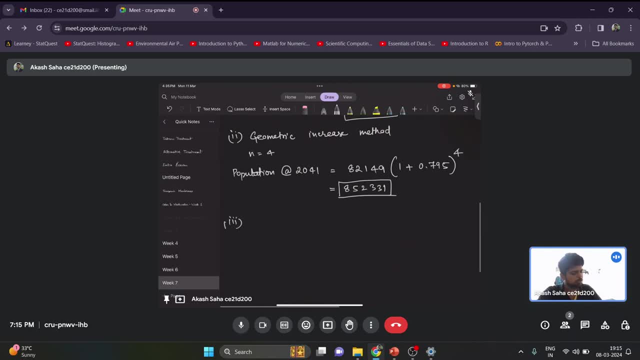 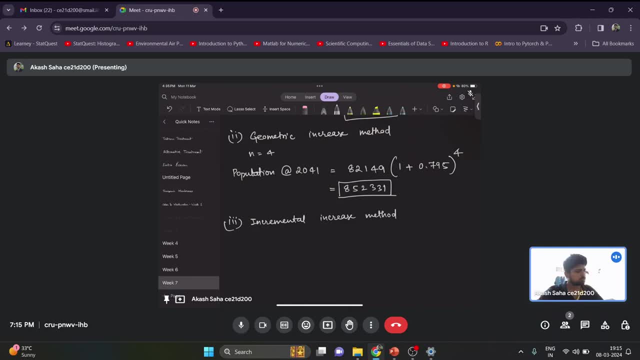 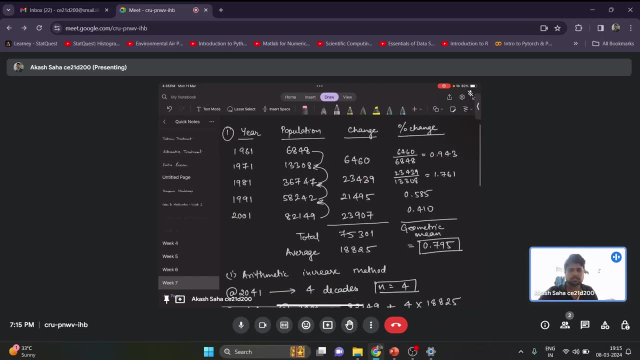 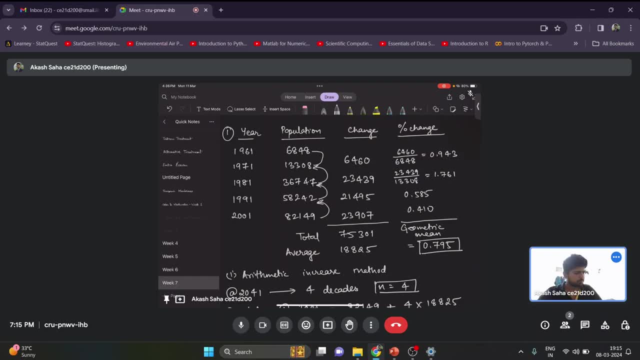 Just take a screenshot of it or write it down again, because I will be using this table again. Okay, I will just remove the percentage change part. Okay, So now, instead of the percentage change, we will find out the incremental change. Okay, 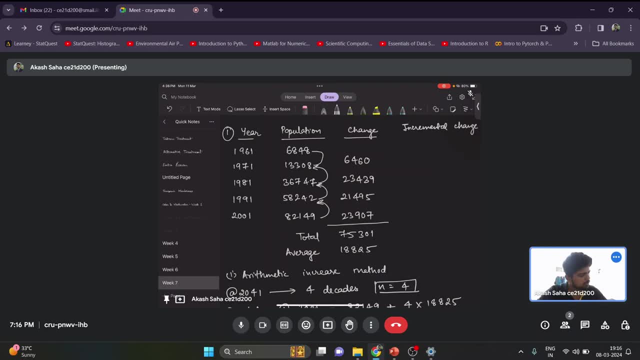 change. so it is nothing but the change in the change column. so again we, we will do what we will do. we will subscribe six, four, six, zero from two, three, four, nine, four, three, nine. so what we will get? we will get something around sixteen thousand nine, seventy nine. again we will. 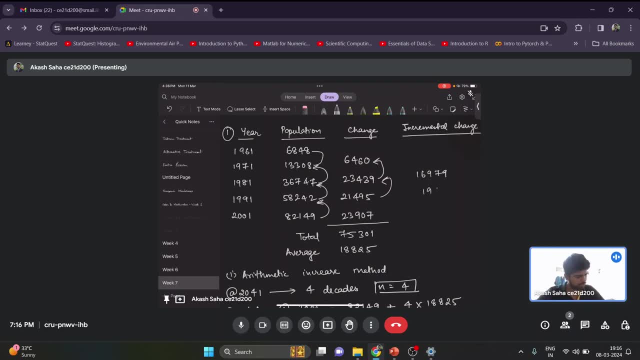 subscribe this from this. so it will be one nine four so, but this time it will be minus and again we will subtract like this, so we will get two four, one two. so this is the incremental changes, change in the change. so if we find out the total, so the total turns out to be something around. 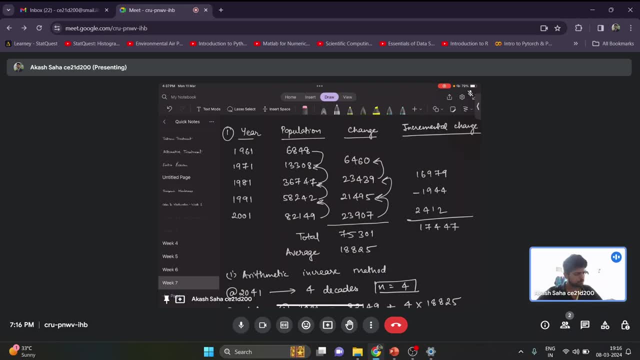 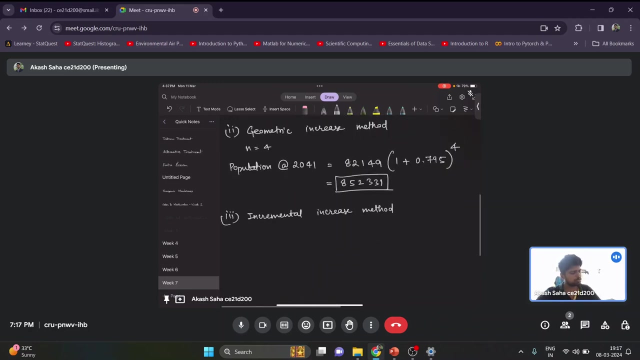 seventeen thousand four, four, seven, okay, and the average turns out to be five, eight, one, six, okay. it's pretty simple. just we have to do subtraction for the change column, so okay, so we'll now see how to find out. so again, here n will be equal to four. 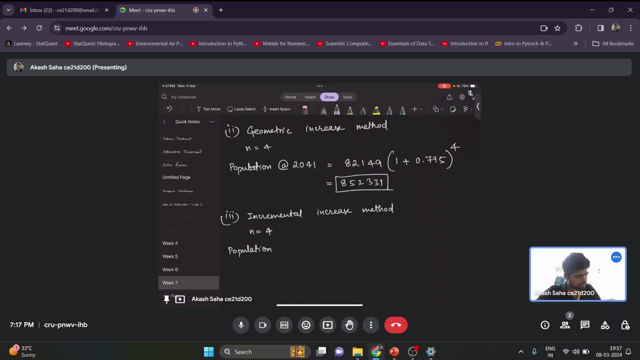 so my population at 2041 would be equal to the known population plus n, and it's four into the average change. so my average change was equal to eighteen thousand 825.. now again, incremental change, for incremental change will be n into n plus one by two. so it 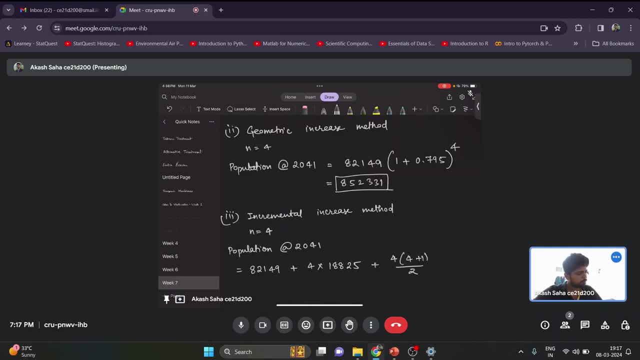 will be four into four plus one by two into the average of the incremental change, so that is 5 8, 16.. into So it will be equal to. so this n into n plus 4, into 4 plus 1 by 2 will become as 5. 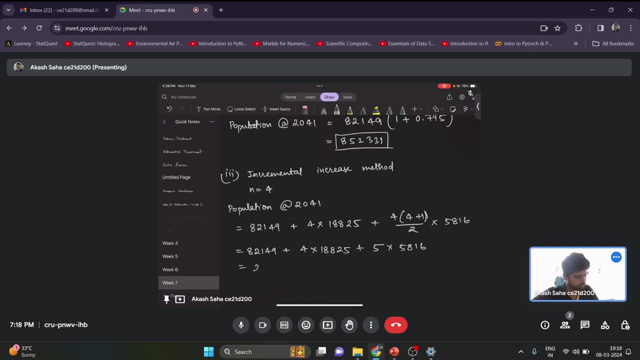 into this. So my final answer will be 215607.. So we can see that the population incrementally, incrementally- is somewhat in between the geometric and the arithmetic. It is considering this extra term here, so this is nothing but n into n plus 1 by 2.. 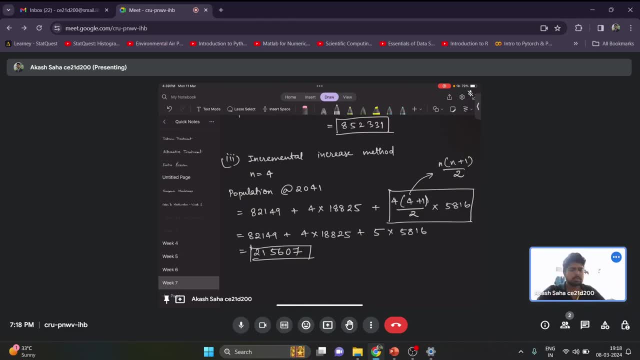 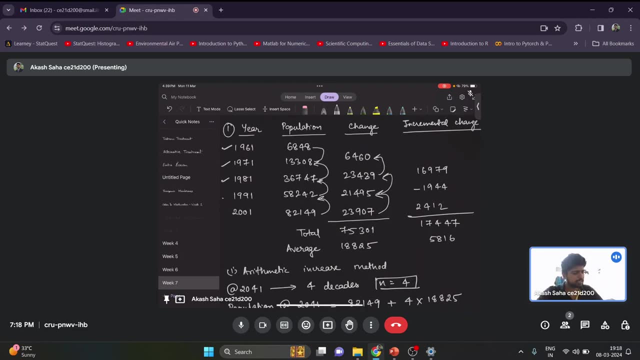 I hope you understood the problem. So I will just finish If we give a recap of this. so you see now the population of each of the decade. so this is the so for the arithmetic equation, you will just find the change. you will just find. 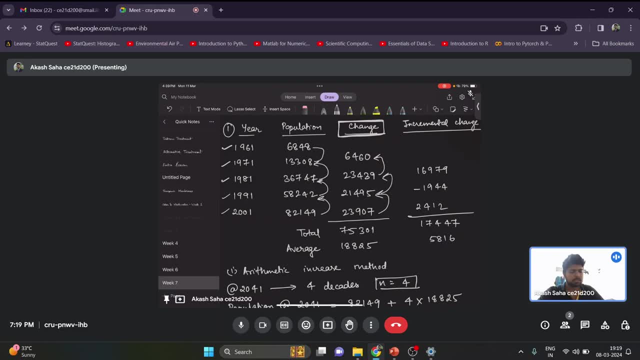 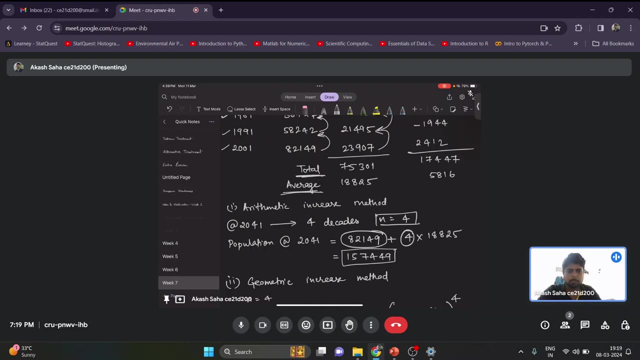 the change. You can just subtract one from the other. you can see the difference in population and then you will find out the total and the total population. So in the case of arithmetic equation method, it is just the last given population. Yes, number of decades for each. in 1 to 1 population, you will see the average. 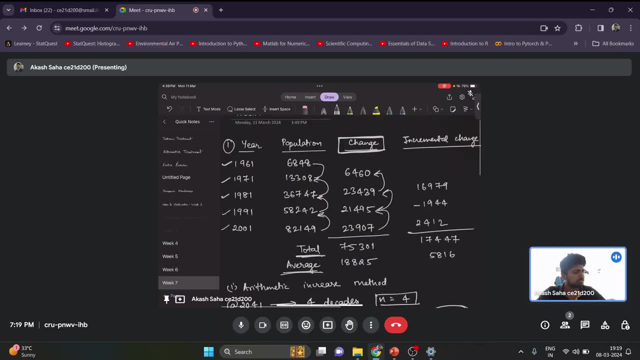 Now, in the case of geometric equation method, you will find out the percentage change. So percentage change for this term here 64006.. So, like that, you will find out the percentage change and you will find out the geometric change. 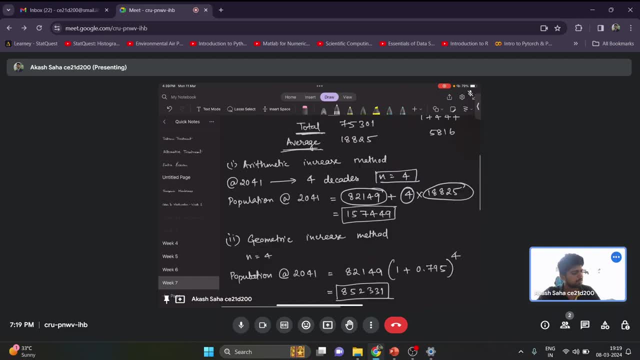 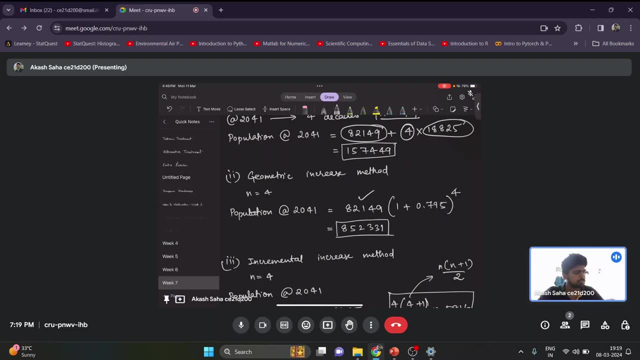 And then, with the help of this, for compound trigonometric formula, the last term that we will draw are just like this: the last time validation, and it was it's value, which is the i and what is the i, so we can get the geometry of the function, and then, in the case of the incremental entry method, we will have two. 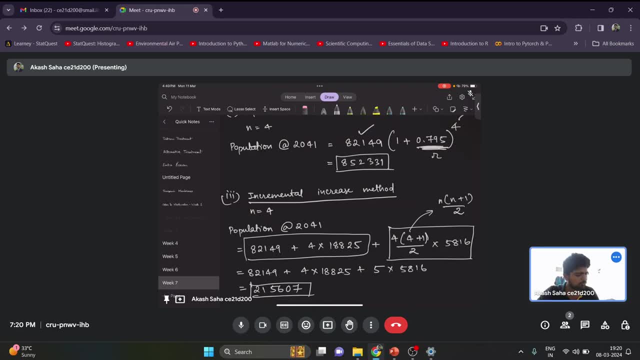 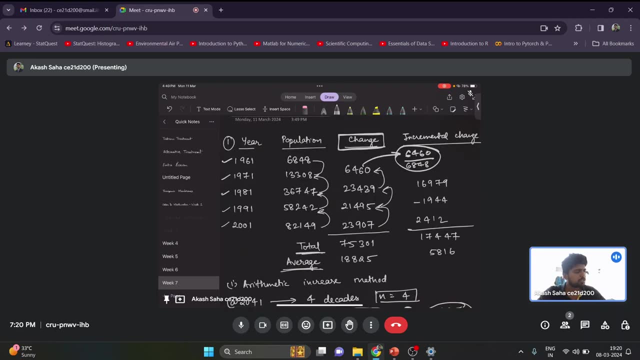 engineers staying in here for the algorithm plus the incremental change. so are you trying to find the implementation? you will first calculate the incremental change for all of these tickets. so here we have to take care of the political navigation, because sometimes the incremental changes can be positive, sometimes it can be negative. so we have to take care of that and 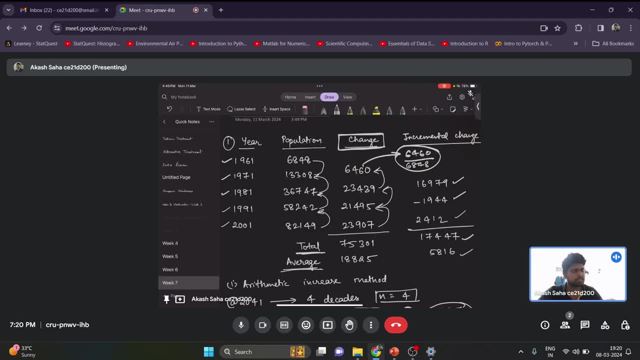 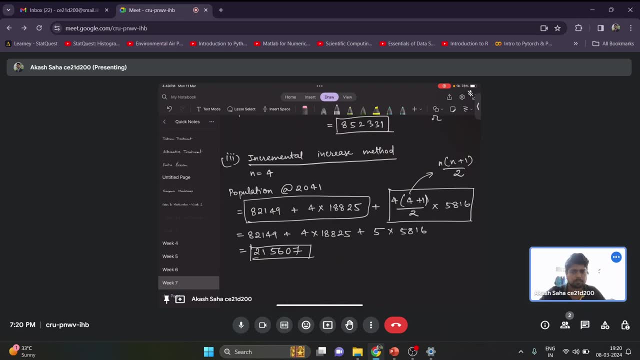 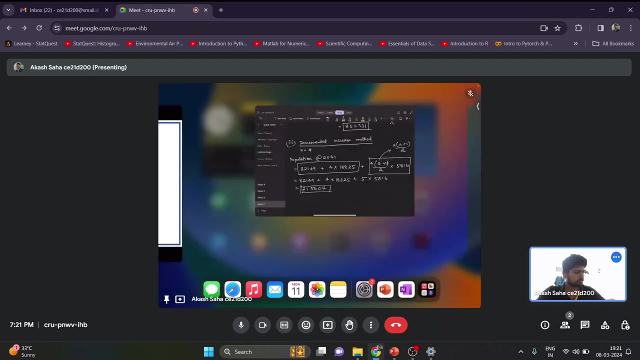 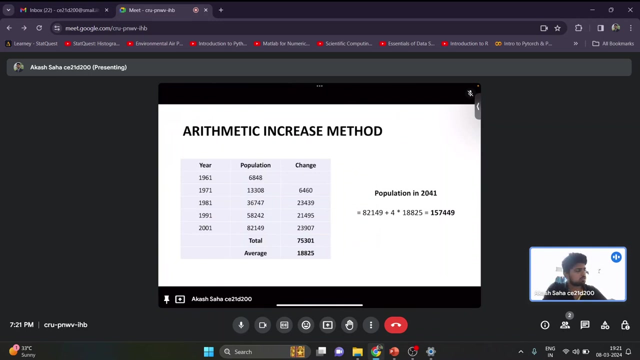 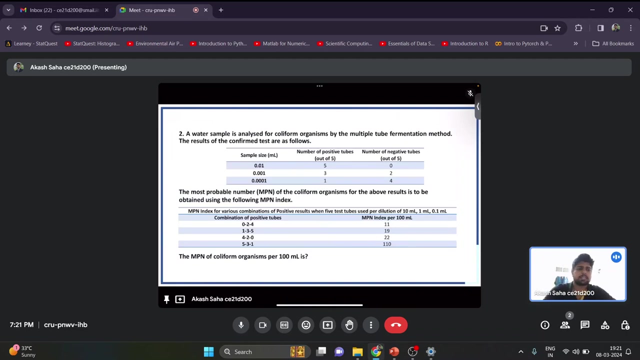 we have to incorporate them in power. there, it's just for you five. okay, now we'll discuss the second problem. so it says that a water sample is analyzed for the reformal visits by the multiple to fermentation method. so the results are confirmed of the control test. 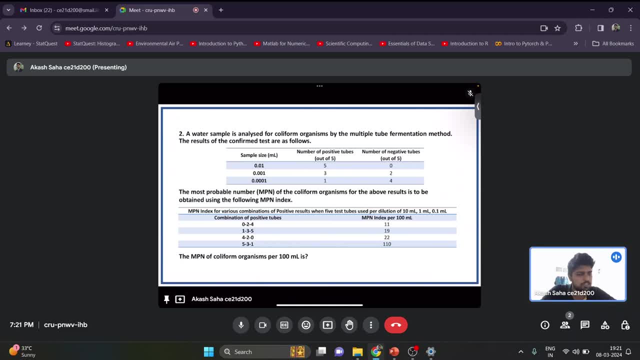 for example in this case, and then the final method is to назыв what we call the night ь the npm, that is the most common number as 35 or 100. okay, so to solve this problem we also need the npm table. so, uh, itself of the npm table is given here, so possible combinations are possible. 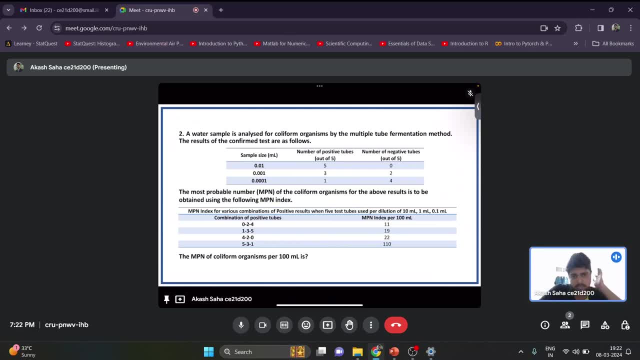 most positive twos are given and the npm is going to handle everything. accidentally, you have much right and you have to solve it to the agenda. okay, so this is the overall question. we'll do it once again and then we will discuss how to solve this problem. 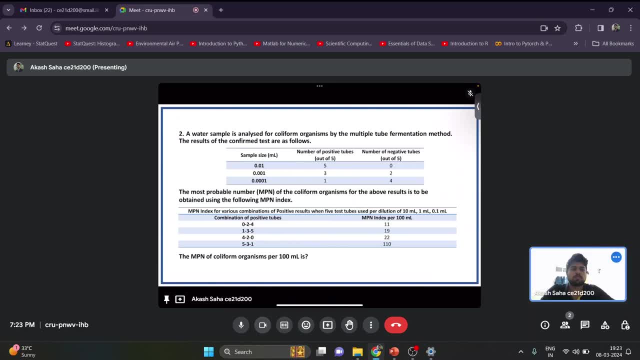 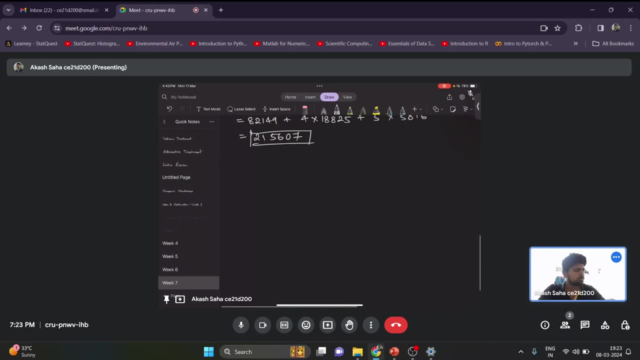 so if you talk about just multiple team fermentation, suppose we have three sets of test strips. so in each set we have five test strips. so each of the test strip we will provide the sample and we will also direct some, or you can say the food for the members. suppose my samples. 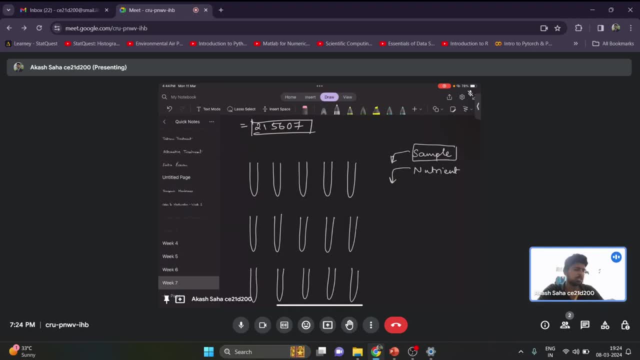 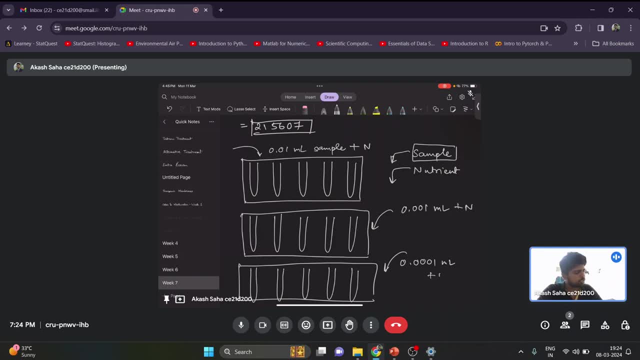 5 meters and movements of flow forward. So after incubating for some various time, we can see there are small error tubes in each of these extremes. These are called inverted tubes. It is nothing but inverted tubes. So if any microorganisms are present, then they are generally designated as a gas solution. 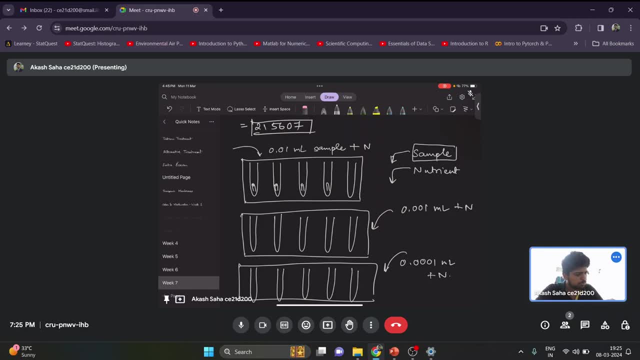 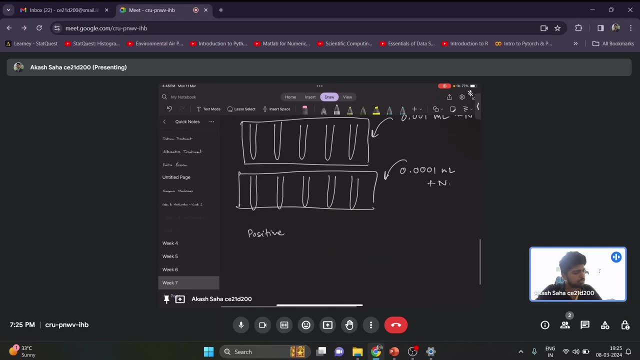 and it will be corrected in this way. Okay, So why the positive speed? So gas in a mix of positive tubes and limited tubes. So the positive speed will be meant to say that gas is gas free. In this case, gas is in the mix of positive tubes and limited tubes. 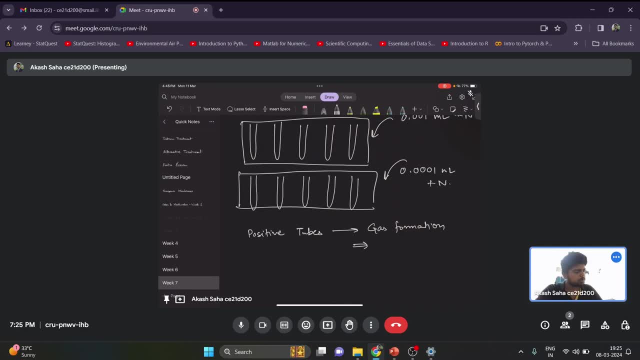 And there will be no showing of gas free in any of these tubes. So relative speed is just like a gas, So it will be consistent. Okay, So these were the two questions which we received, that if any microorganism is present, 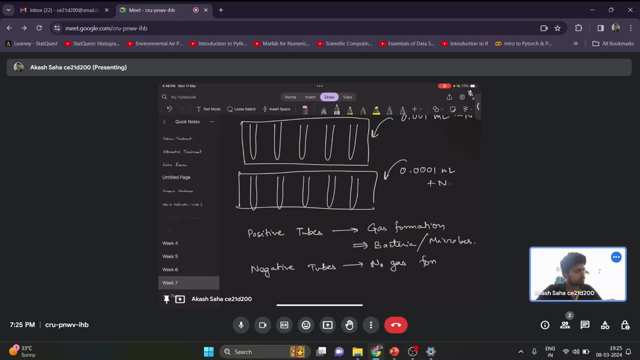 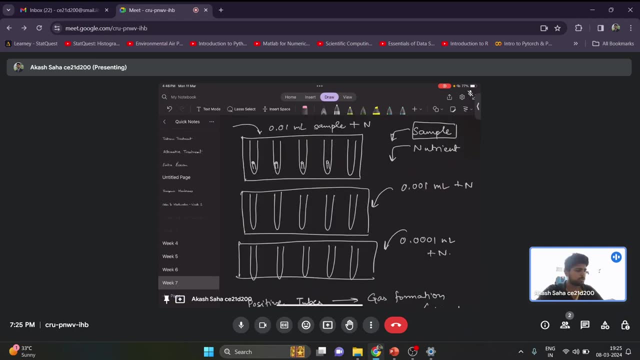 then some bacteria or some microorganisms will occur And in negative tubes there is no gas free. So what? the question says That on the side of 0.001%. So all of them have got yes. for the next set, we have 3 positive case and the next set. 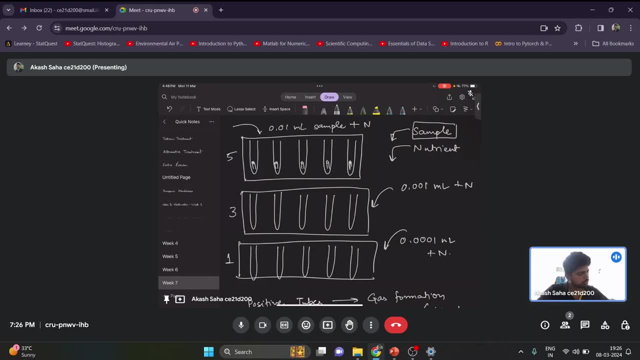 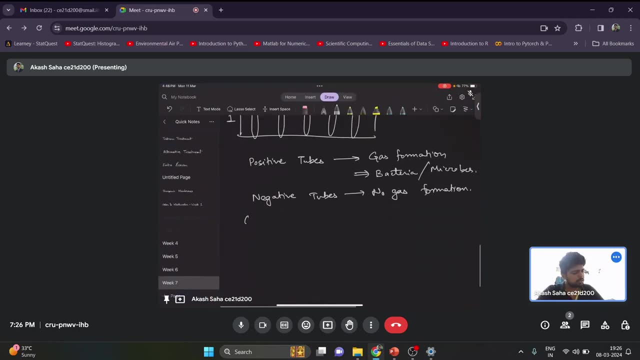 we have 1 positive case, So 1,, 2,, 3,, 4,, 5,, 9,, 10,, 11,, 12,, 13,, 14.. So if we see the combination of positive case, we are getting it as 5,, 3,, 9,, 10,, 11,. 12,, 13,, 14,, 15,, 16,, 17,, 18,, 19,, 20,, 21,, 22,, 23,, 24,, 25,, 26,, 27,, 28,, 29,, 30,, 31,, 32,, 33,. 31,, 32,, 33,, 34,, 35,, 36,, 37,, 38,, 39,, 40,, 41,, 42,, 43,, 44,, 45,, 46,, 47,, 48,, 49,, 41,, 42,, 43,. 42,, 40,, 42,, 43,, 44,, 45,, 46,, 47,, 42,, 43,, 44,, 45,, 46,, 47,, 50,, 51,, 52,, 53,, 54,, 55,, 56,. 57,, 58,, 58,, 59,, 60,, 61,, 62,, 63,, 63,, 63,, 64,, 57,, 61,, 62,, 62,, 63,, 64,, 57,, 62,, 63,, 62,. 62,, 62,, 63,, 62,, 62,, 62,, 63,, 62,, 62,, 63,, 63,, 62,, 63,, 64,, 64,, 65,, 67,, 67,, 69,, 68,. 68,, 69,, 69,, 70,, 71,, 71,, 72,, 72,, 73,, 71,, 72,, 73,, 72,, 73,, 72,, 73,, 72.. 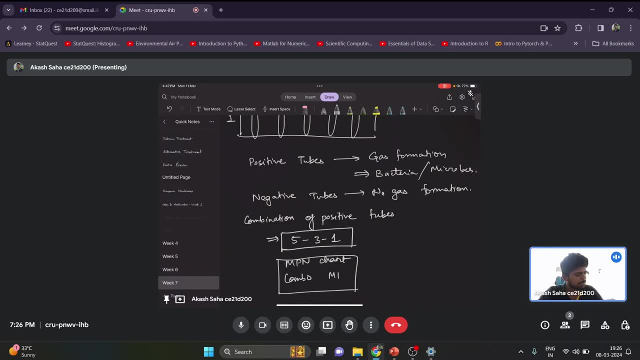 So if we see the NPN chart, on the left side there will be this combination and on the right side there will be NPN. So for this size 31 combination we have to see the corresponding one. So for this size 31 combination we have to see the corresponding. okay, so that chart. 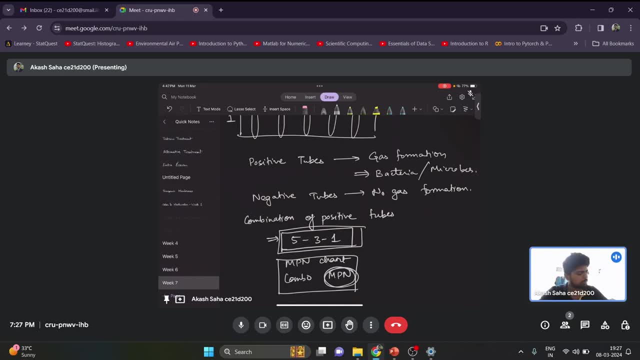 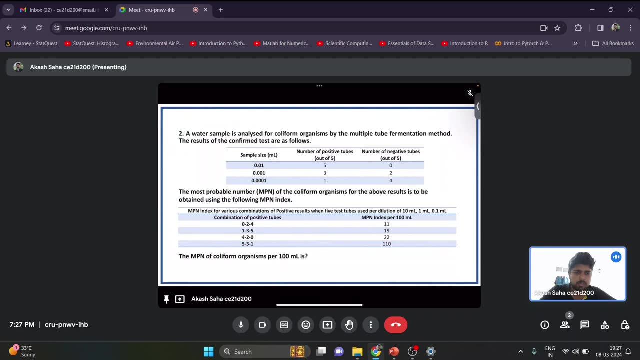 must be available with the chart size so you can see the chart. so in this chart we can see that corresponding to size 31,. okay, the NPN index is 100, the NPN index is 110 and one might say that the answer of this question is 100, but that is not the case. 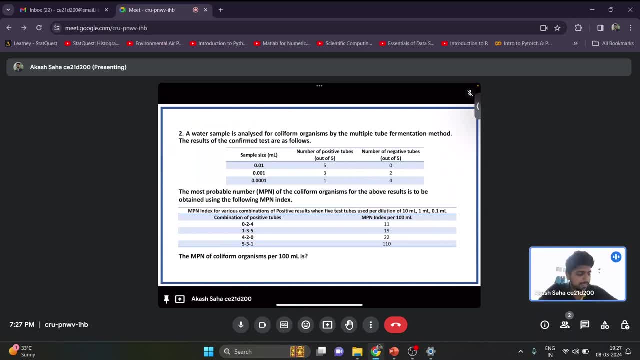 we have to take care of one more thing Now. this NPN index chart is given for the combination of those different units when the test tubes used for dilution is of 10 mm variable and 5 mm. Okay, so for this sample size of. 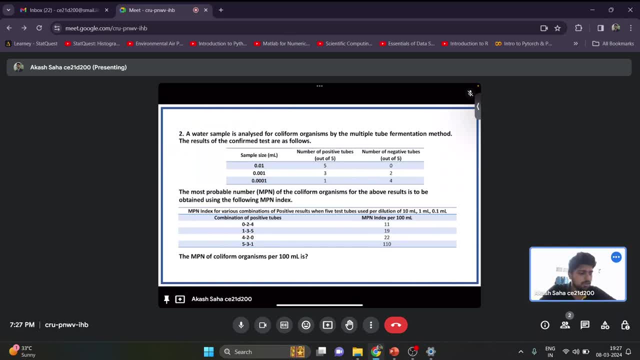 10, 1 and 0.1,. this chart is given, but in our question the sample size which we have taken is 0.01, 0.001 and 0.0001, so there is an order difference of 1000, because instead, 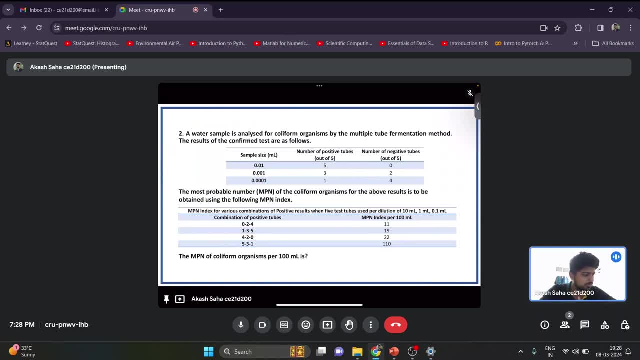 of 10 mm. we have taken 0.01 as my first sample. So there, if we divide 10 by 0.01, we will get 1000, so there is an order difference of 1000.. So once we have given, we have to simply multiply this area difference with our continuous 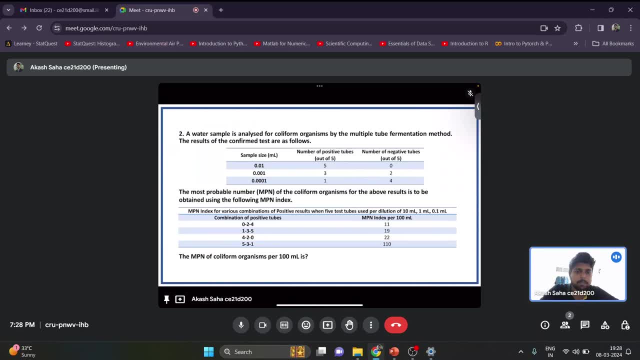 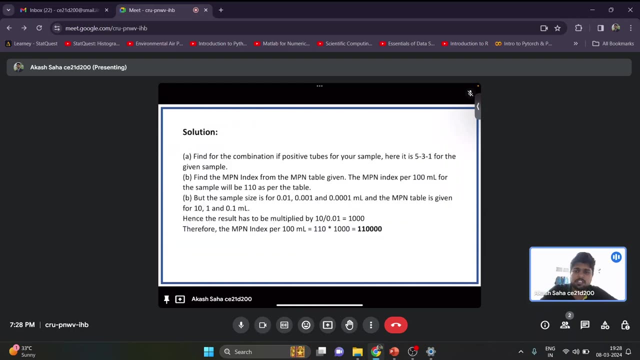 So for 5,, 3, 1 combination, NPN index is 110, now there is an order difference of 1000, so we multiply by 10 to 1000, so we will see the function. So at first we have to find the combination of positive 2s of our sample. so here it is. 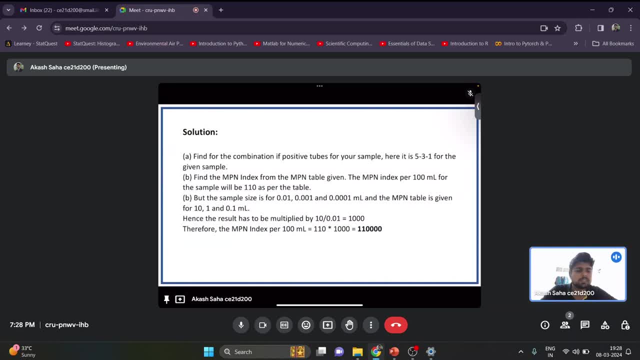 5,, 3,, 1.. Now find the NPN index from the NPN table. So for 5,, 3,, 1, the NPN index is currently like this: Now what the sample size is for 0.01, 0.001 and 0.0001, what the table is given, so 10,. 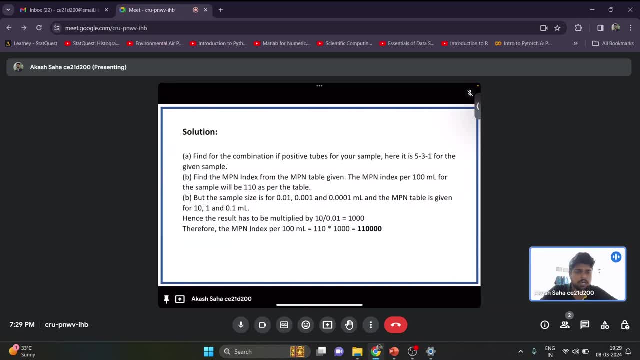 1, 0.1.. So the order difference is 10 by 0.01, which is 1000, so we will simply multiply the NPN index. Okay, Now, if we maximize. so now, right there it is. 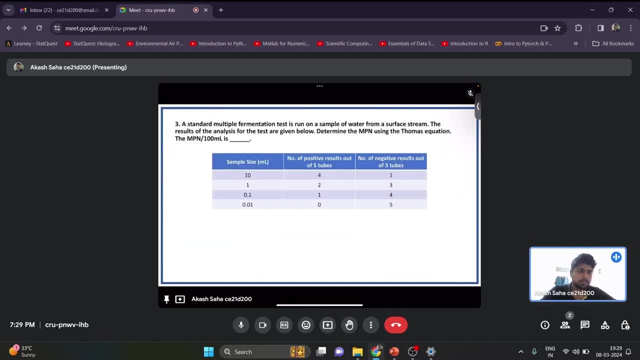 And then we get the sample in 22.. So the sample as it is and 0.01, 0.01.. So it is divided equal to its limit. 2. related to the multiple fermentation test. so it says that the standard multiple fermentation test. 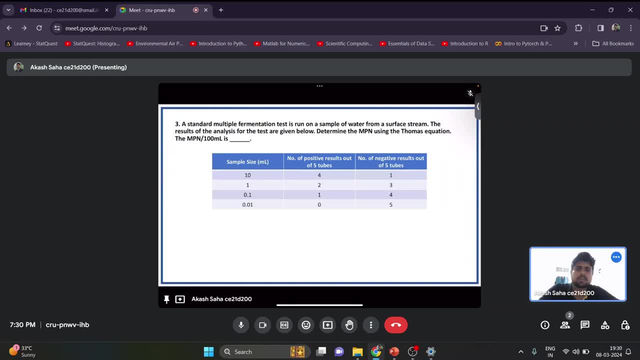 is. there are one sample of water from surface stream. the results of the analysis from the tests are given below. determine the entry using the thomas equation. okay, so here you have to use the thomas equation. so again, the sample size is given. we have been given the results and the number. 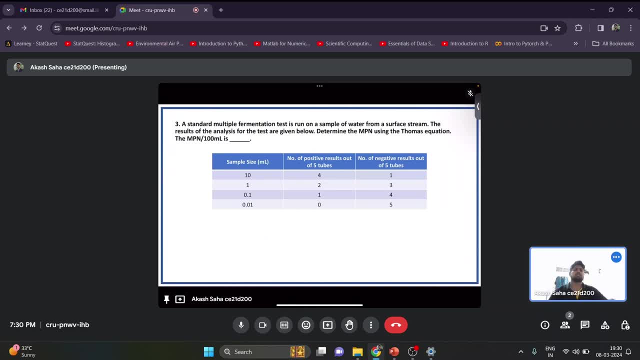 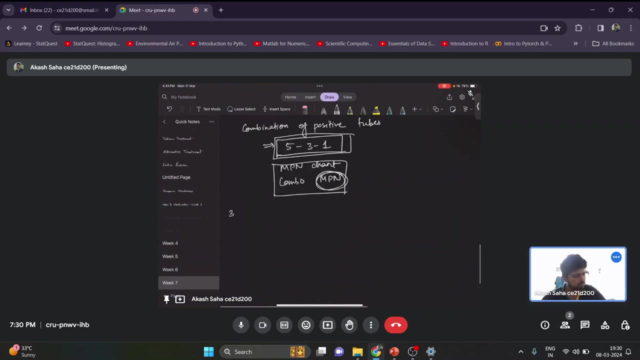 but we have to find out and build the thomas equation. we will see what is the thomas equation and how we have to find out. we just need to note all these questions, okay, so that we can solve it and solve this right. so now the thomas equation. so if you see the thomas equation, 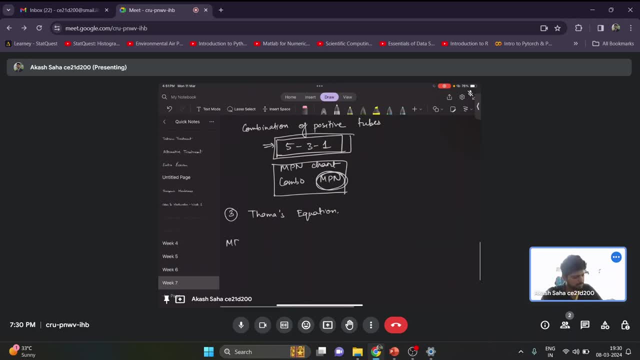 is something like this, and here divided by square root of okay, and then of sample in like it is, and in value of sample again fine. so this is the equation for the thomas evaluation. so what is the number of positive? so the number of positive is 4 plus 2 plus 1. 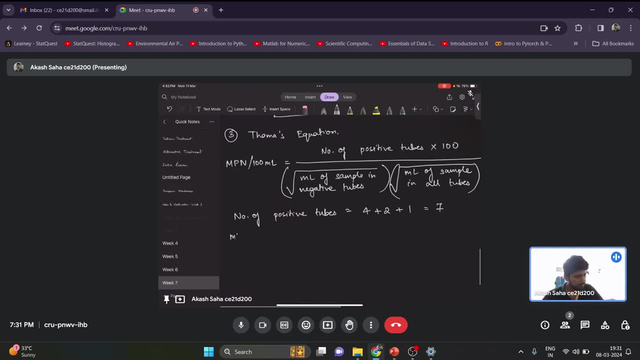 this is the sample. okay, now ml of sample in negative streams will be 1 okay into 10 plus 3 into 1 plus 4 into 0.1 plus 5 into 0.1. so this 10 1.1010. 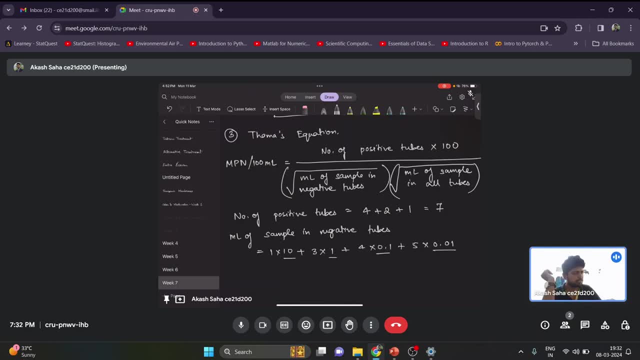 by sample. so since in the first set four were positives, so one will be okay, then two were positive, three will be negative, one was positive, four will be negative, then zero was positive, five will be negative. in like that we have 10.0, so that means we will give it around 1.1. 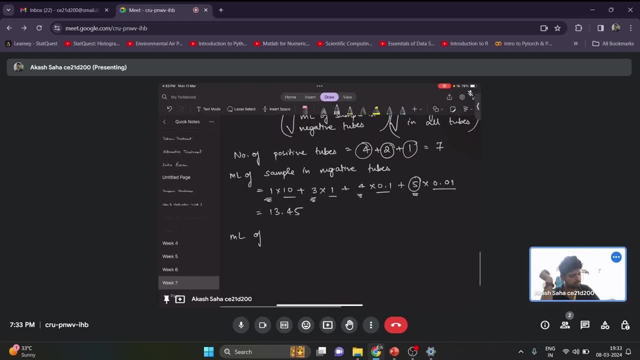 plus 1.0 and then we will find out the values. all samples: okay, so it should be. so it should be in the upper left: 5 into 10. okay, and 5 into 1, 5 into 5, 5 into 1, 5 into 2. 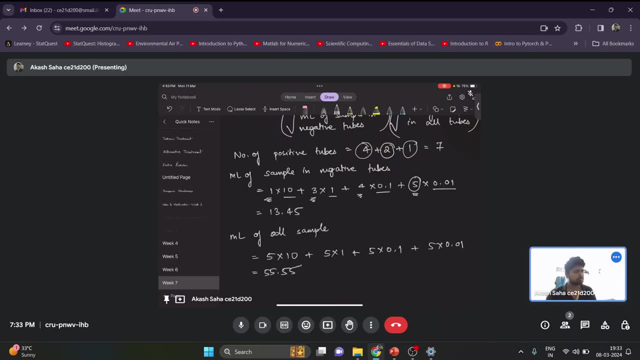 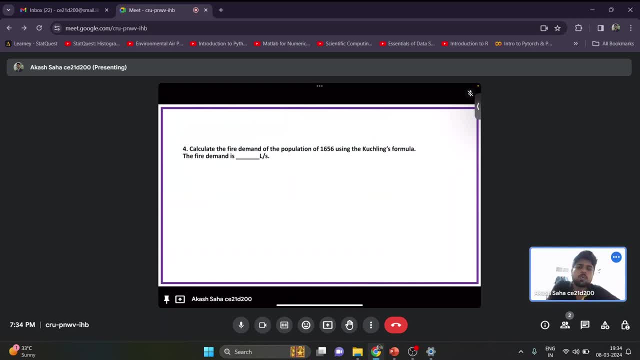 yes, ae. So we have 1656 using the Cuchling Simulator, the Simulator documentation to clear up the code. So now we use the Cuchling Simulator, we come to the final part. So here we have to take care. we have to take care of the anti-guidance. 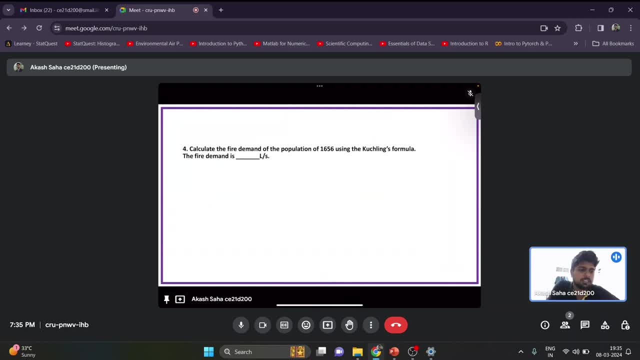 So we have to take care of the anti-guidance, which is only for moving, for example, to the right side. Here the demand is: has it been used in the first situation, Just to make sure that it looks like it's not there? 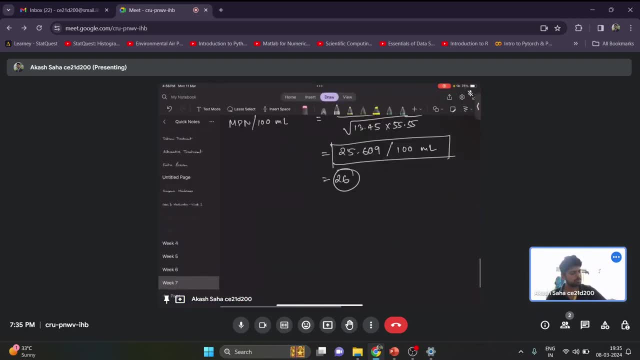 So if you see the Cuchling Simulator for final removal, Okay, So for final removal, it is very straight forward. Okay. So here the fire demand. okay, the question is, you want it to be pretty comfortable, but here the fire demand is very little. 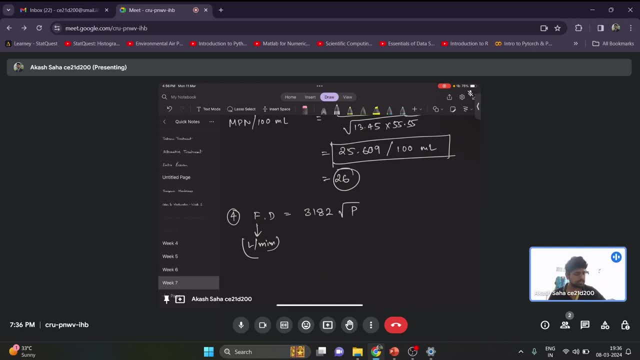 Okay, It's. it's a direct formula, So you have to take care of the movements. E should be the population of the region, but we don't know the size of it. We are going to take care of the size, We are going to take care of the equation, but we are not going to take care of the size. 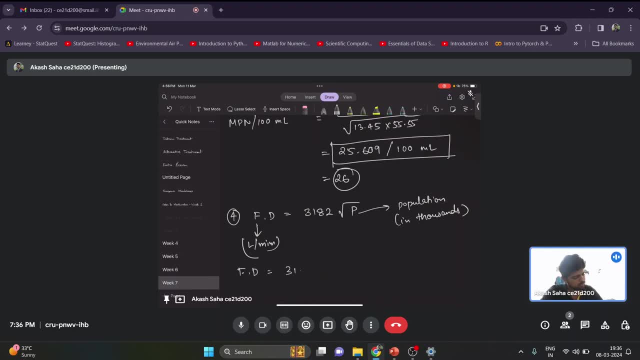 So my FD is 1656.. Before E was 1656. But that is 1656. So we are going to charge it 1656.. So now I am putting it on my S and I am going to collect it and send it to the source. 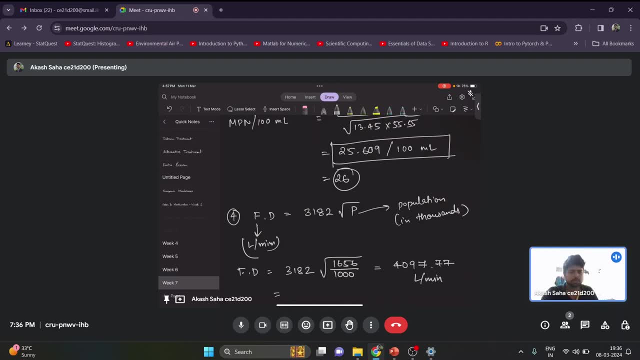 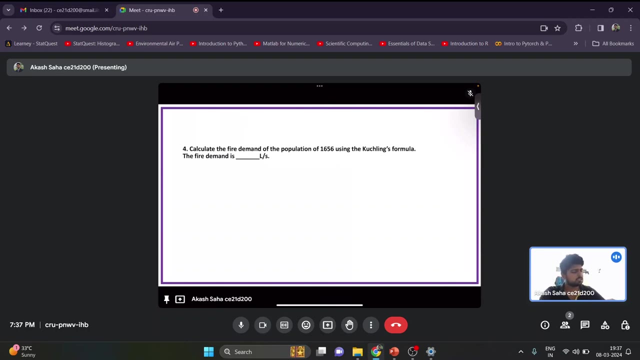 I'm going to do that one right here. So here is where I am going to send E to safety. I have two operations here. The first is I am going to sign E to safety From there. you have two operations to sign E to safety. 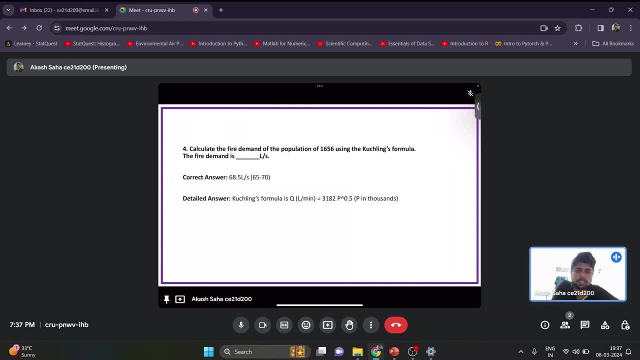 And when you complete sign E you win in litre per minute is given as 318.2 kW. So we have to manage the solvent type. So we have given four categories: chemical, central, biochemical and biological. Which category do we need to respond to in large quantity? 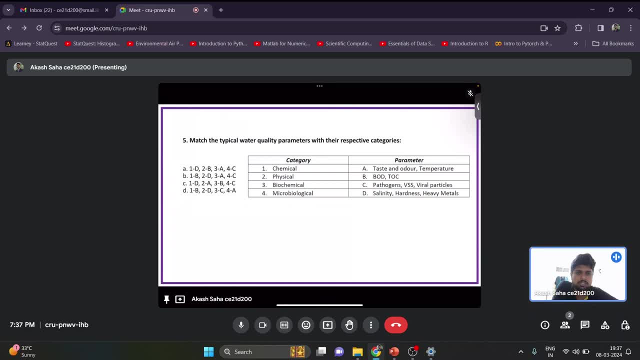 So the options that we have. Let's try to go to the next slide. Okay, So for chemical category, we have the salinity and hardness of the chemicals, because these are chemical properties of matter, And then, for physical, we have the resistance of the temperature. 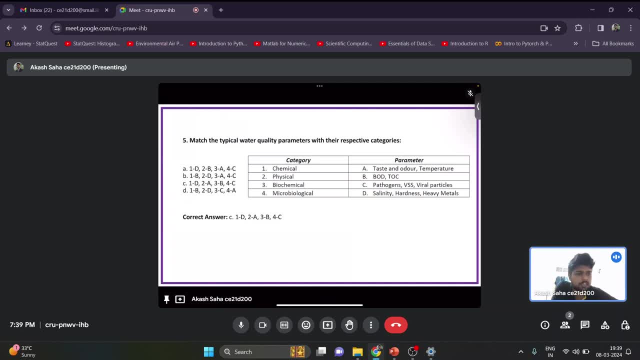 So for biochemical we have the CO2 and CO3. We can add biochemical oxygen to that. And then for the microbiology we have the percentage of pathogens. that validates the spin-off values and the non-validating values. So the percentage of the valiant process, of the spin-off values, are a measure of the 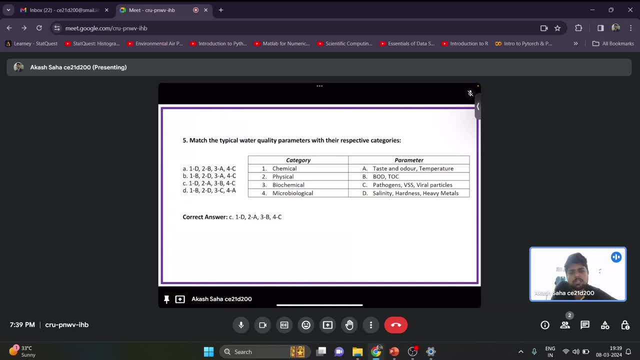 non-validating values, as we've seen in the video. So we just match the current kind of degree. Thank you, Thank you. So it says that this Zeta potential, which is the electron potential, is shared in the particle surface. 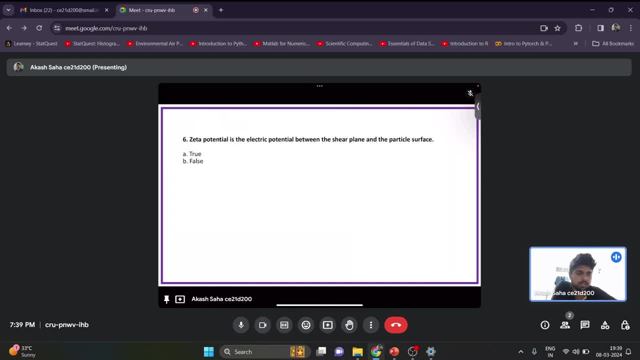 So it's true. Yes, So the gravitational changes, the wavelength of the electron potential which has to be overcome. So that's true, Because the as it can be measured. So it says that for the Zeta potential, it's the electron potential which we can measure. 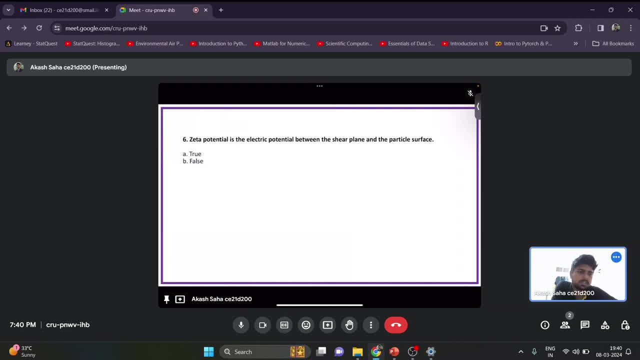 It will eventually become the shield of change. Just think about it. It's true, It's happening. The correct answer is false, Because the vector potential is the electrical connection between the shear plane and the bulk solution. It is not the particle sequence. 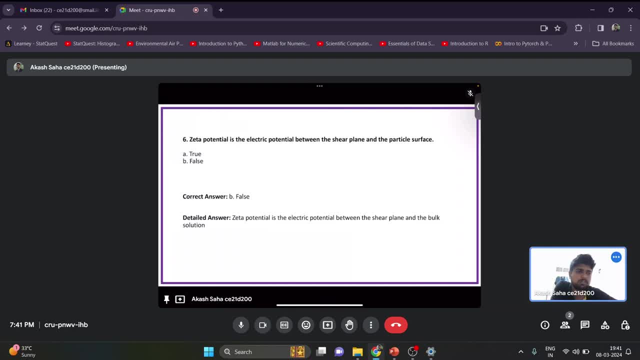 It is the bulk end solution. Okay, The particle sequence of the solution, The potential difference between the shear plane and the bulk solution, And the potential difference between the shear plane and the bulk solution. It's clear, It's true. It says: select the correct characteristics of the bulk solution. 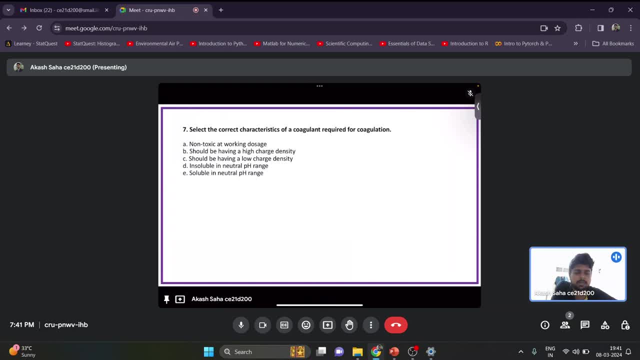 The bulk solution And the characteristic characteristics. Now we get a correct answer, okay, So you can see the statements one by one. So it says non-toxic at working dosage. So 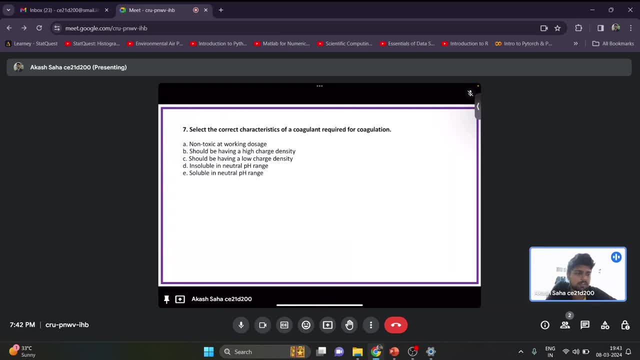 a coagulant must be non-toxic, Otherwise there is no point of using that coagulant. And then talking about the charge density: the charge density is very high for a coagulant, So option B is also correct, that it should be having very high charge density. 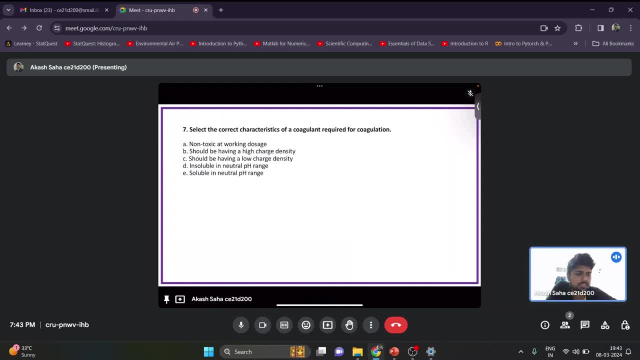 And if we see the performance at neutral pH range then it should be insoluble. But because if it is soluble then again there is no use of a coagulant. So the correct options are A, B and D. So it should be non-toxic at working dosage. It should be having a high charge density. 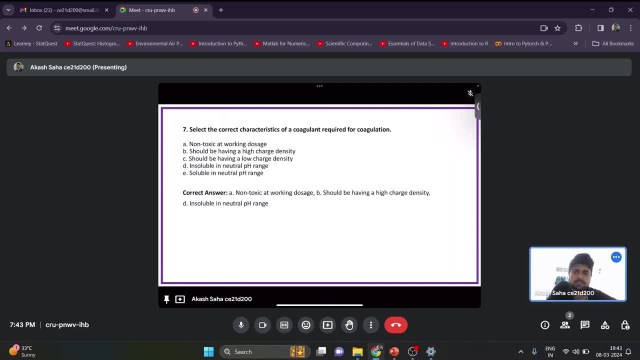 And it should be soluble in the neutral pH range. So this was the seventh question. Now we move to the next problem. Now it says that about coagulation theory. the net force on the colloids is repulsive at greater distances and becomes attractive. 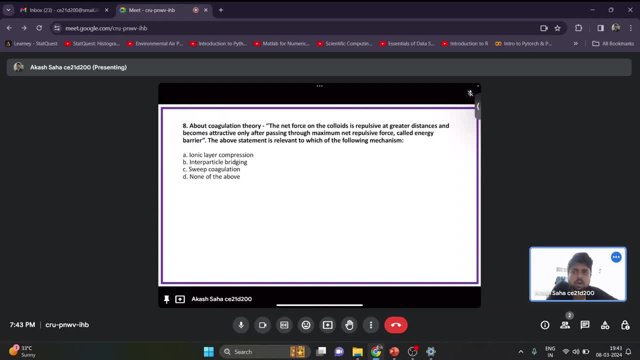 only after passing through maximum net repulsive force, called the energy carrier. The above statement is relevant to which of the following mechanics? Is it ionic layer suppression, Inter-particle bridging, Seed coagulation? None of the above. So, again going through this statement, it says that the net force on the colloids 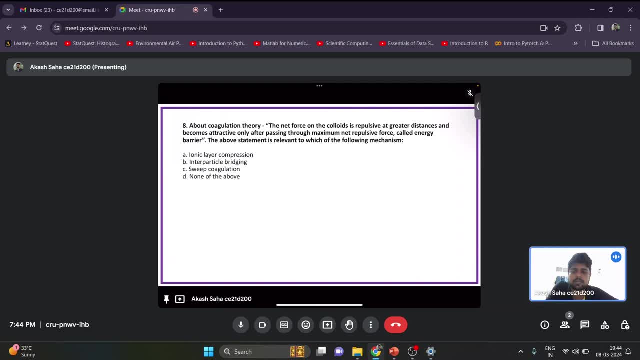 is repulsive at greater distances and becomes attractive only after passing through maximum net repulsive force, called the energy carrier. So this is relevant to which of the mechanics? So we have learned about four absorption mechanisms. three are mentioned here. Other one is the absorption and charge neutralization. So for which of the following? 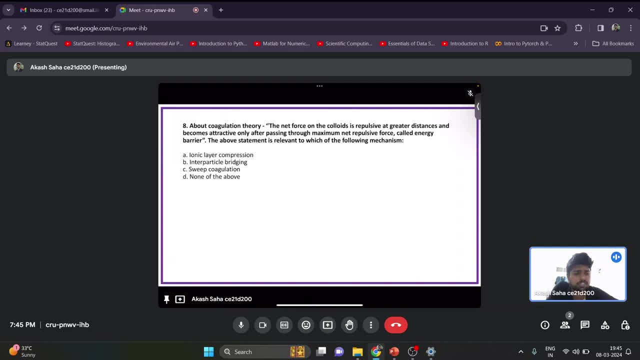 it is true. So, as you see, in the case of only ionic layer compression, the net force on the colloids has to be very, very important for getting the best стали compression. It has to overcome the distances and so that the attraction sources 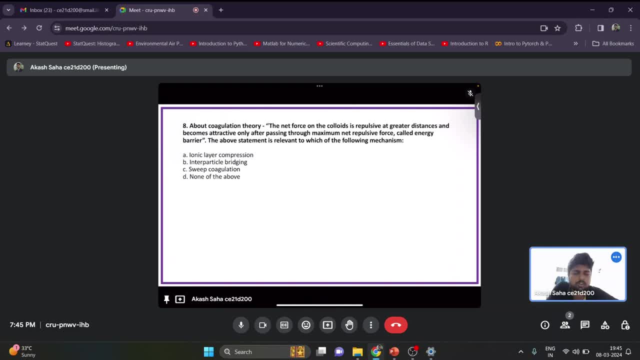 are more so that the particles can come together and then settle down. So in the case of only ionic layers- compression- this theory holds true and it is relevant, Not holds true. it is relevant, Whereas in the inter-particle imaging it is just in the long change polymers, how the particles 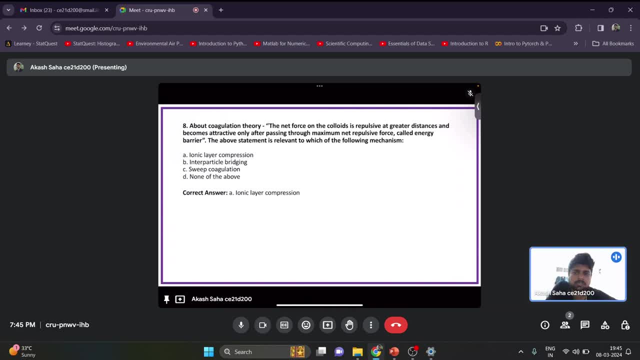 are getting attached, and same case in the case of silk curvation, how the gelatinous slots are formed, like in the case of alum or AL3 case. So the mechanisms are different. whereas there is a repulsive and adaptive source concept, in the case of the ionic layer compression, the option A is correct. 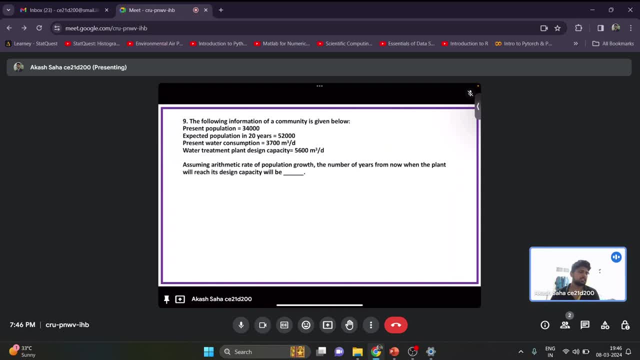 Now again, I follow the medical. it says that the following information about the community is given below: The present population is 34000 and the expected population is 20 in 20 years is around 50,000 and the present water consumption is around 3700.. 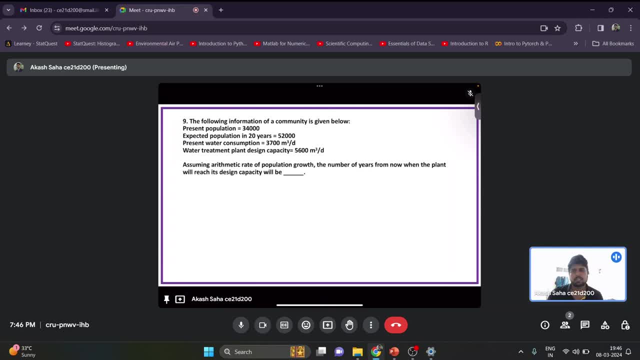 Okay, Okay, 300 meter cube per day and the treatment and the plant capacity for which it is designed is 1500.. So we have to assume arithmetic rate of population growth and find out the number of years from now when the plant will reach its designed capacity. 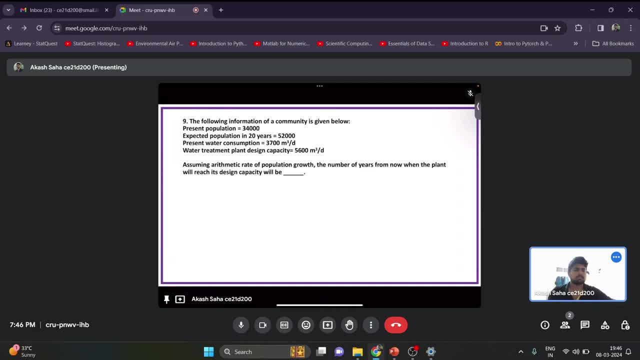 Okay, So the present and the expected and the projected is given, So we have to find how many years, in how many years So the community will reach that designed capacity. Okay, It is a simple problem. just try to understand it. go through the problem once again and 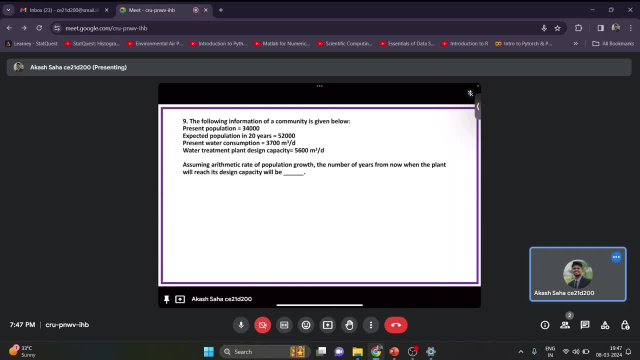 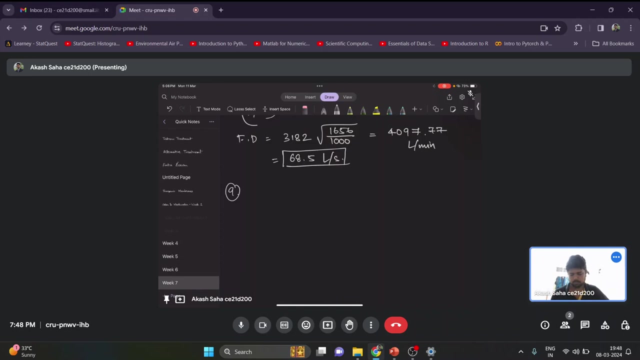 they will reach the same. Okay, Thank you, Thank you, Okay, so we'll see the solutions. So the present population is around 35,000 and the expected population is around 55,000.. So if you find out the average increase of population per year, say 20,000 to 30,000,. 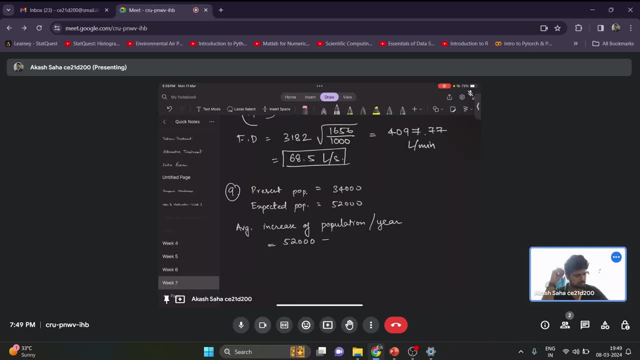 it will be minus 24,000 divided by 20, because this expected population is given in 20 years, But divided by 20, so my per year population increase will be around 925.. Now the present water consumption, if we see it, is designed for 3700 meter cube per day. 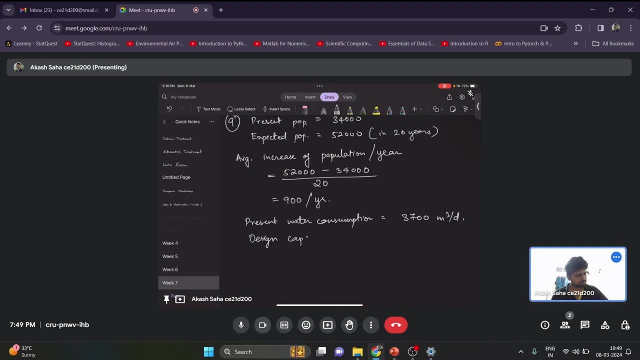 and the design capacity. and the design capacity is 5600 meter cube per day. So we So we calculate the average max capacity So it will be around 5600 minus 3700. So that is around 1900 meter cube per day. 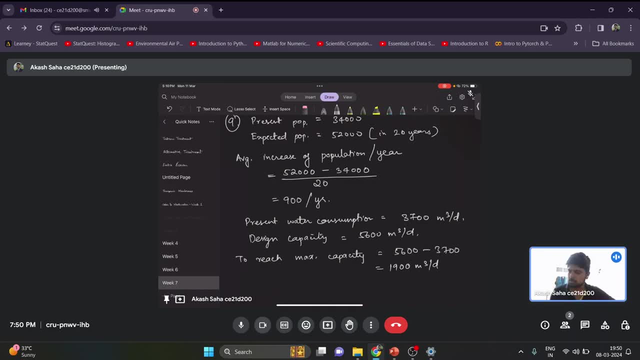 So more 1900 meter cube per day of more water consumption can increase. Okay, so this is the difference. So now, if we calculate the present average water consumption per head per day, So per capita or per day, how much water is being consumed? if we see: 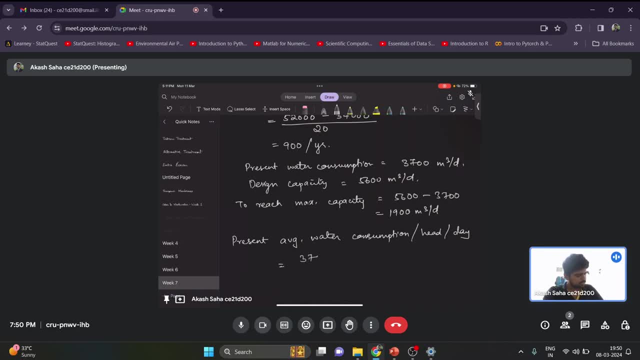 So the total water consumption is 3700. divided by the population of the present, that is 34,000.. So it will be around 0.1088.. Okay, So this much amount of water per head per day is required. Okay. 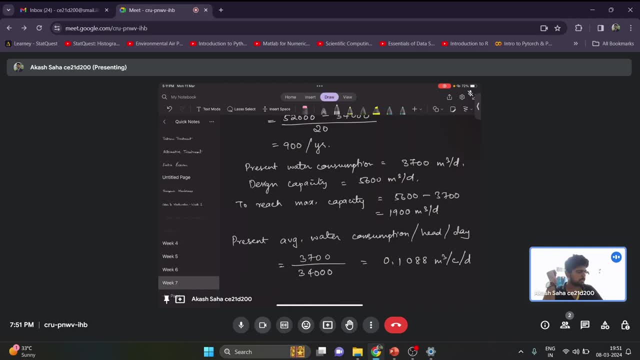 So meter cube per capita per day. So now we know that per year 900 people are increasing, So increase in consumption, Okay, Okay. So it is about 0.1088 meter cube per day, So the total consumption of water. 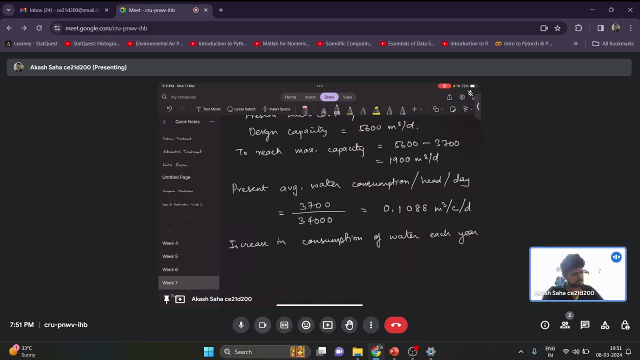 So in each year how much consumption is increasing? So we will simply multiply 900 into 0.1088.. So it will be around 97.9411 meter cube per day. Okay, So this much amount of water consumption, Okay. 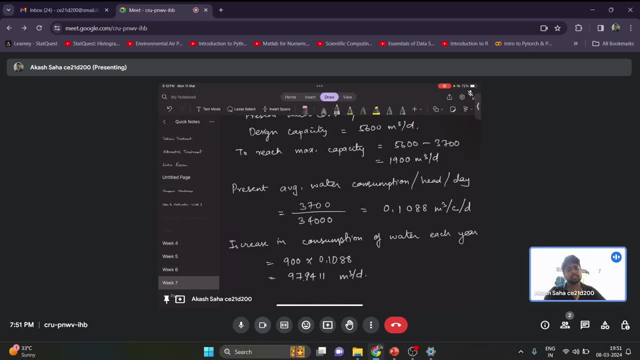 Okay, Okay, meter cube per day is increasing per year, So in how many years it will reach the design capacity? So number of years to reach the design capacity will be the difference between the design capacity and the present thing, that is, 1900. 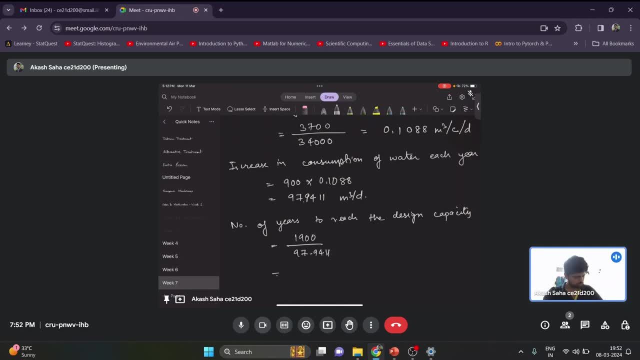 divided by 97.94 water, So it will turn out to be 19.4 years. So in 19.4 years it will reach the design capacity. So this is the water content, Basically nothing. Just you have to find out like how much will be the increase per year of population. 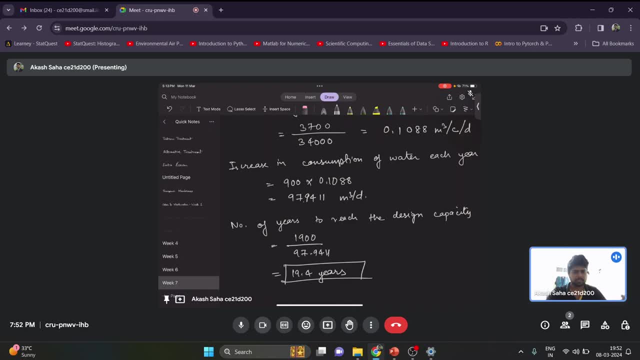 How much of the water consumption difference is still present. what is the per capita use now and per year? how much increase will be there? and then the number of years to find to reach the design capacity. So it will if it is around 19.4 or around 20 years. so this was the overall problem. 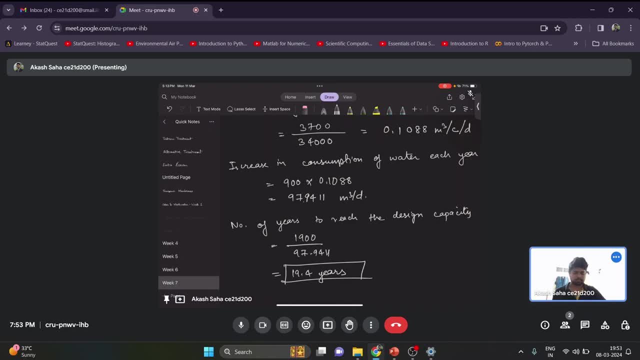 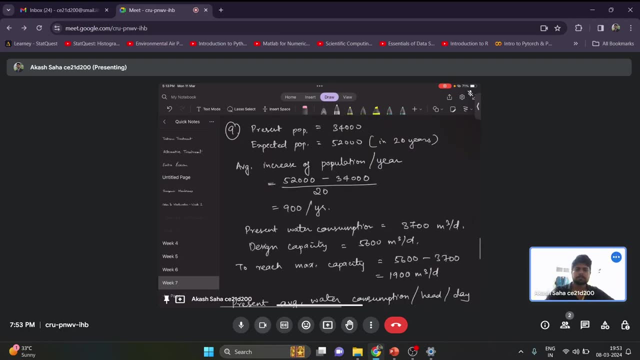 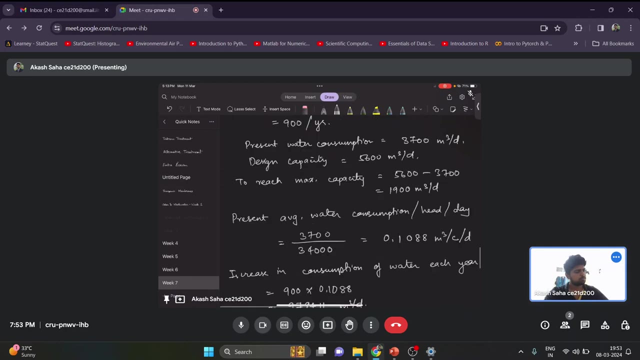 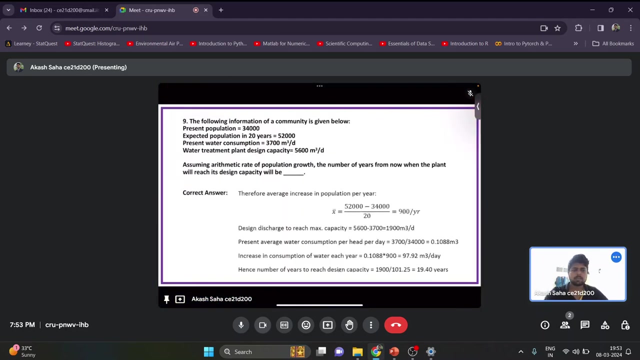 I hope it is clear to all of you. If you want, you just can go through it once again, right? ok, so this is the answer. you can also add it here. you can check the PPT letter, Ok, So the next question now: compute the fire demand for a city of 1.5 lakh population by. 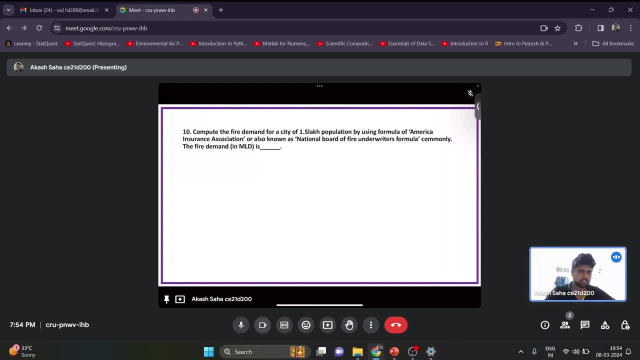 using the formula of America Insurance Association, or also known as the National Board of Fire Underwriters Formula, commonly. So we have to find out the fire demand and the answer should be in America. Ok, Just try to recall the formula for the National Board of Fire Underwriters, or it is also known: 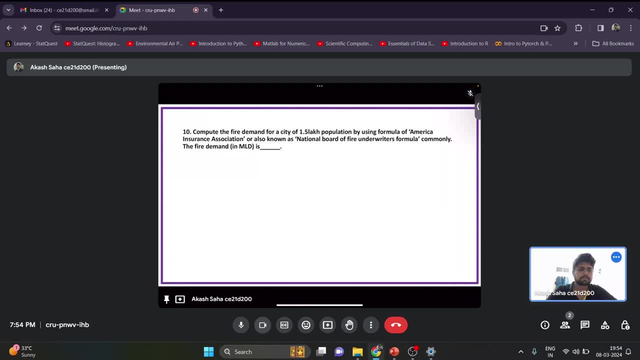 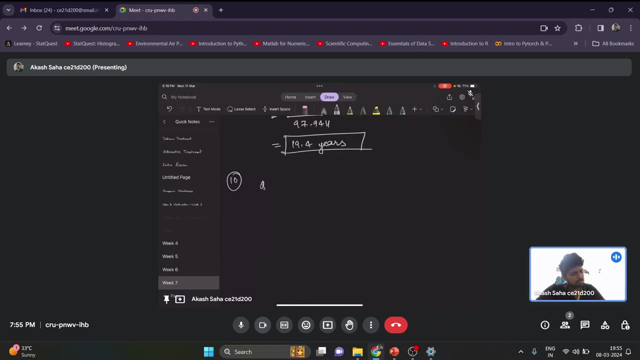 as America Insurance Association. Ok, So, Ok. So I have found this. Ok, You will see the formula for this. So the formula is given as Q in liters per minute is given as 4637 under root p into 1 minus 0.01 under root p. 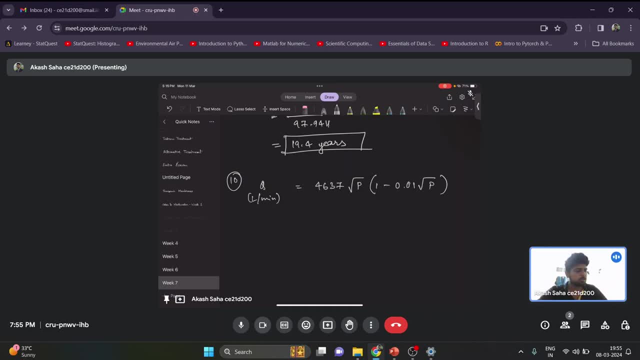 So again, the discharge here empirically is found out to be in liters per minute and the p is the population in thousands. So again the same funder in thousands, you have to find out. So it is given for 1., 1.5 lakhs, so in thousands it will be 150. 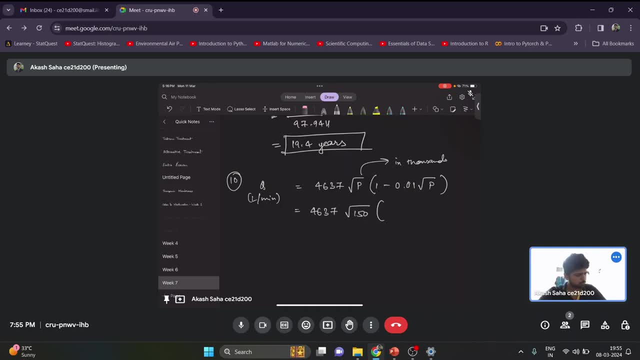 So 4637 root 150, 1 minus 0.01 root 150, so it will turn out to be 4985.9 liter per minute and in MLD it will be 71.7363.. So you have to report the answer in MLD. 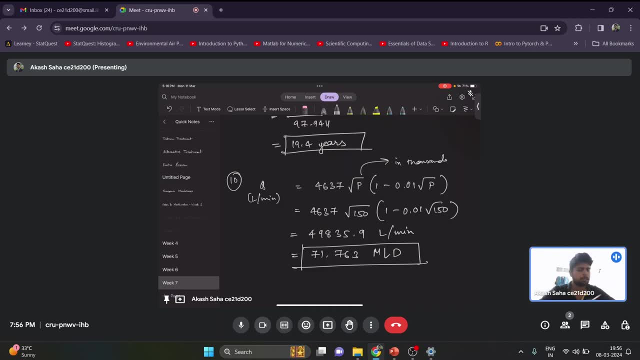 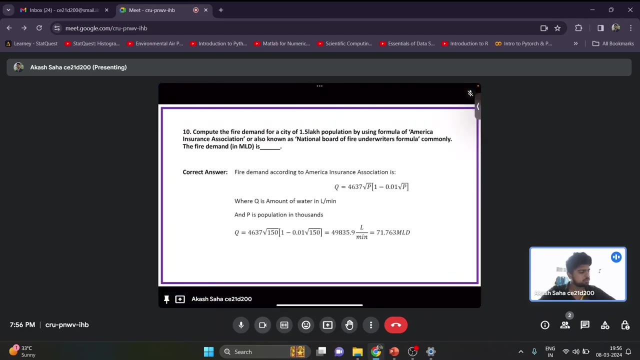 So it will be 71.763.. So it will be 71.763.. But the actual answer will come in liters per minute. so just you have to take care of that. So I have put it clear. it is a very easy and direct question. 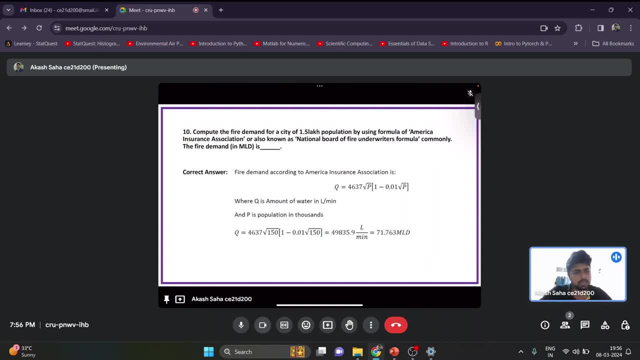 So this is the answer: 71.76, around 72 MLD will come. Just make sure that you are putting p in thousands, that is, the population in thousands, and the final answer is in 1000.. So this is the answer. 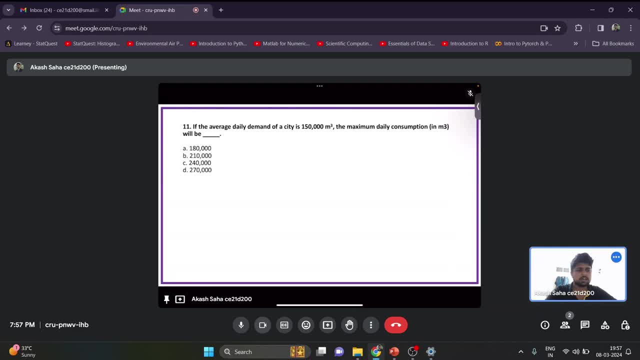 So this is the answer. So let us talk about what we can do. So the next problem: the average daily demand of the city is 150,000 meter cube. maximum daily consumption will come. So here we have to make use of the peak factors or the other daily, hourly and weekly factors. 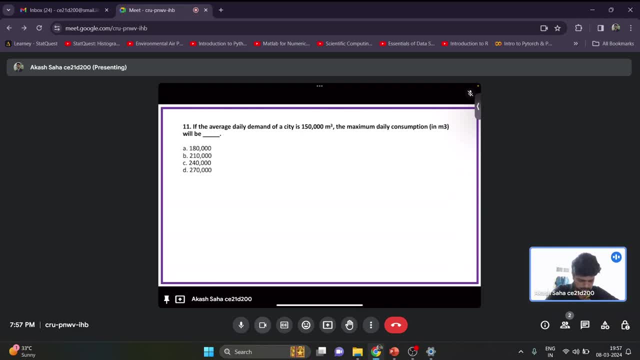 So the average daily demand is given, What is the factor that we have to multiply? So the correct answer is 270,000, because the factor that we use, as for the daily variation factor, is 1.8.. So, from average daily demand to maximum daily demand. if we have to find out, we have to. 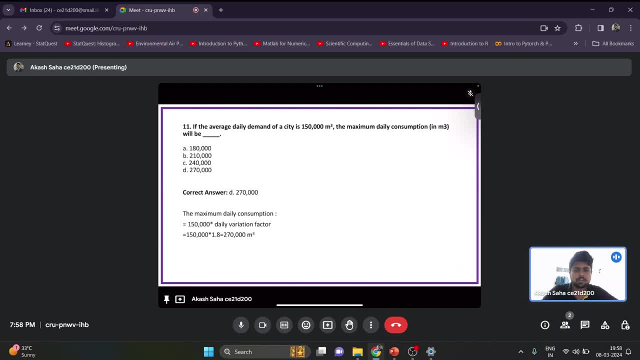 multiply it with the factor of 1.8, so 150,000 into 1.8 is 270,000 metric cube. so this is the answer. We will move to the next problem: match the typical water quality parameters with their. 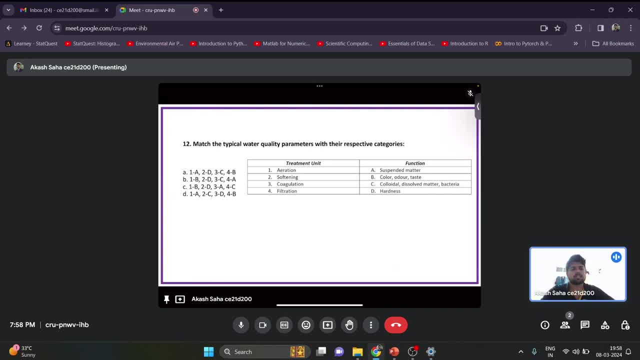 respective categories. So again, we have a treatment unit and the respective function. So we have aeration, softening, coagulation and dilution. So what different functions do they perform? we have to match with them. So please try to find out. go to the question once again, and then we will discuss. 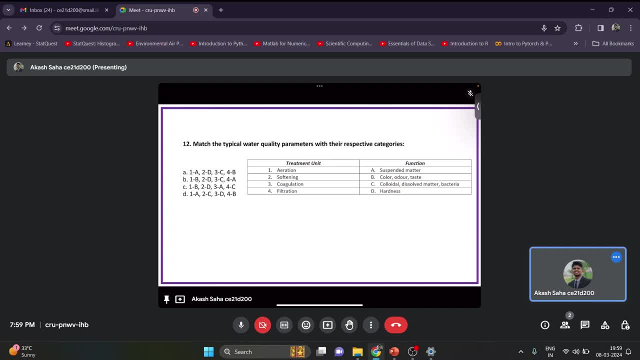 Thank you. So if we see here, the aeration unit will be used to remove the colour, order or taste. The softening unit is obviously for the hardness, where we have to remove them, And then the coagulation unit can be used for the suspended matters. 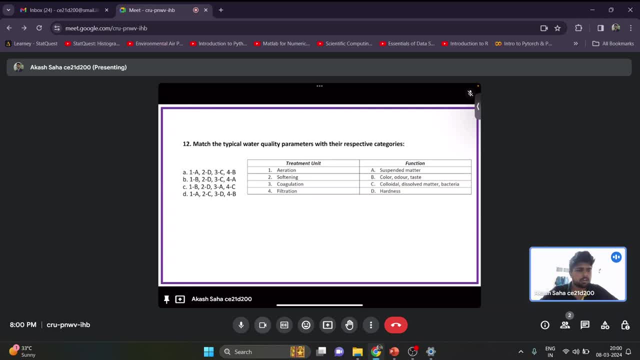 And then the filtration unit can be used for the colloidal dissolved matter or the bacteria. So if we match all this, we will get the answer as C, 1B, 2D, 3A and 4C. It is very simple. 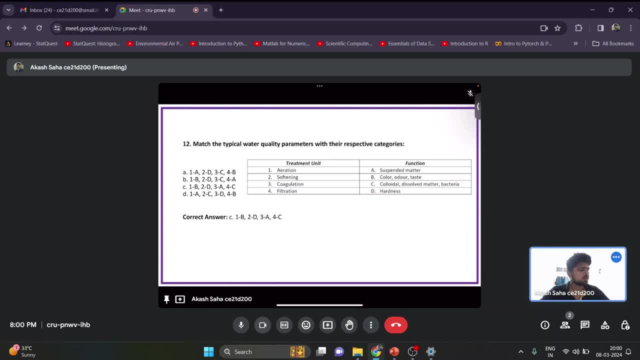 I think you can make out easily The next question. Select the correct statement Regarding the coagulation. So it says that alum coagulation produces aluminium hydroxide flocs in flocculation process. Alum coagulation decreases pH in water. 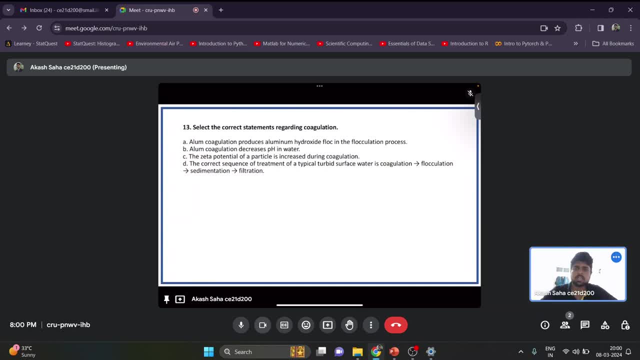 The zeta potential of a particle is increased during coagulation and the correct sequence of treatment of a typical turbid surface water is coagulation, flocculation, sedimentation and filtration. So four statements are given. We have to find out the correct answer. 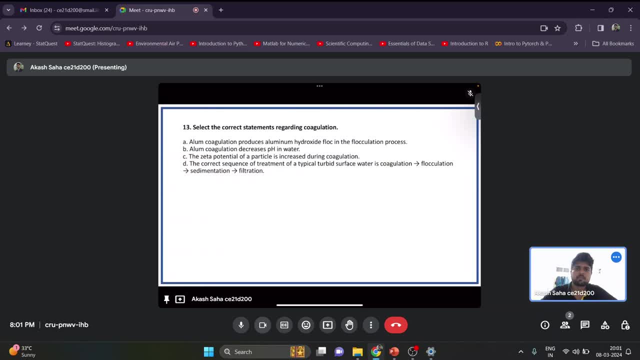 Okay, Thank you, Shabana見. Did we get that right? Yeah, Thank you, Yeah, Yeah, Okay, think here, as far as the answer is concerned, only one of the statement is incorrect. So if you see all the statements one by one, so alum coagulation produces aluminium hydroxide. flow. So that is true. And also alum coagulation decreases the pH, because we know alkalinity is directly related to the alum coagulation. it takes up alkalinity, So it will decrease the pH. So option B is also correct. Now the zeta potential of a particle is increased. 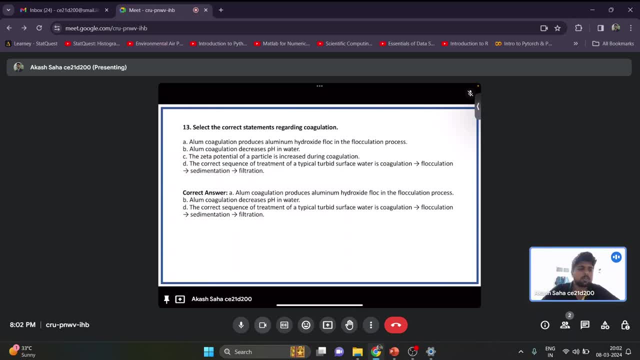 during coagulation, which is not true because the zeta potential will be decreased in the case of coagulation. So option C is incorrect And the other thing, the correct sequence. it is also signed because after coagulation it goes on flocculation and then sedimentation. 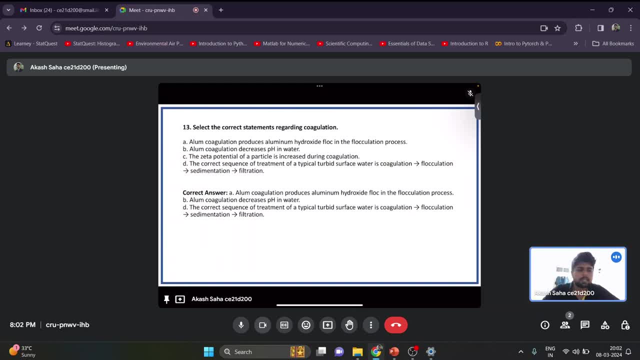 and fibrillation respectively. So option A, D and D, all are correct. So this was about the 13th question. So, except for the C statement, because the zeta potential will be decreased during the coagulation process, So option C is incorrect. Move to the next problem. 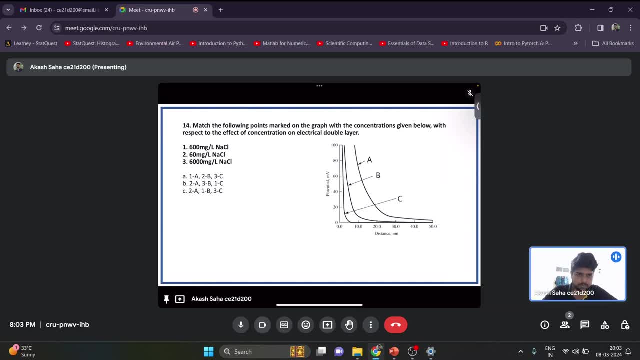 The following points are marked on the graph with the concentration given below with respect to the effect of concentration on electrical double layer. It is talking about the electrical double layer. So we have three different concentrations of magnesium: 600 milligram per liter, 60 milligram per liter and 66000 milligram per liter. So we have to find out. 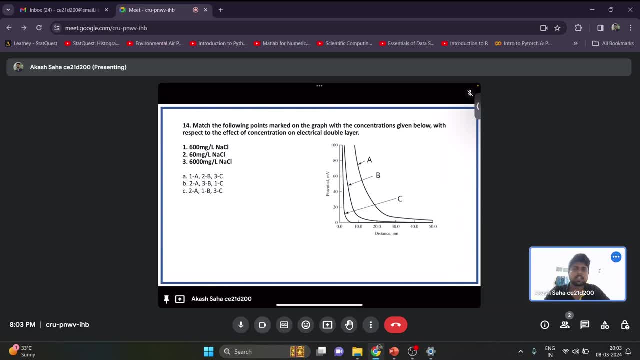 the correct option, which is depicting the effect of concentration on the electrical double layer. just have to see the distance of the electrical double layer. So if you see the curve will move closer to the y-axis or the distance will reduce If more and more particles or concentration is there. so in that case the farthest away. 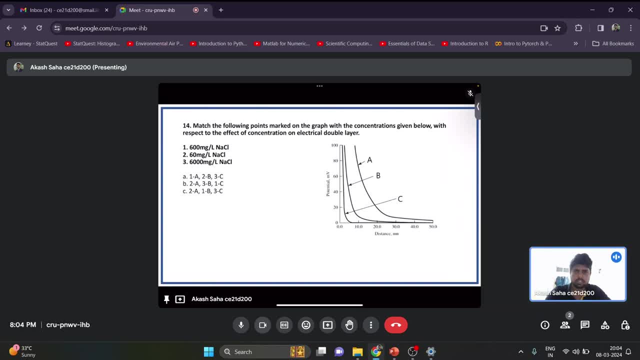 will be the least concentrated particle of the solution. So we can say that 60 milligram per liter of NaCl- that is, the second option- will be the A curve, because this is the farthest away. So the correct answer is C, that is, 2A, 1B and 3C. 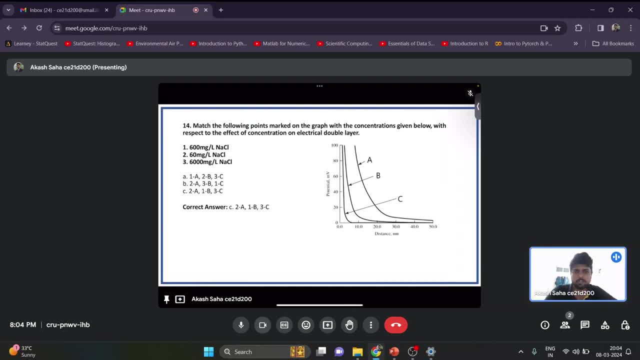 So 60 milligram per liter will be the farthest away. Then in between we will have the 600 milligram per liter and then the closest to the y-axis. that is, the least distance is for the third or with the maximum concentration, that is. 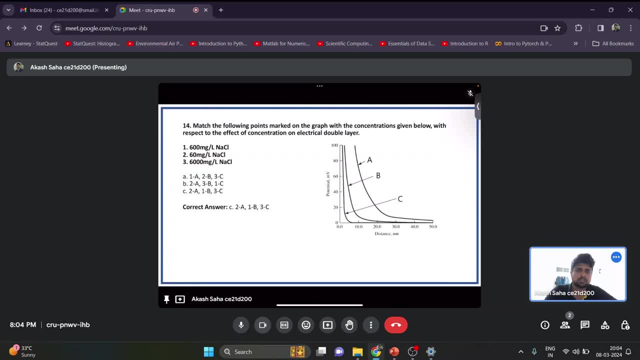 the 6000 milligram per liter. So this is the correct option for C. We will move to the next problem now. In a water treatment plant, the optimum time of flocculation is 0.5.. This is usually given as 30 minutes. 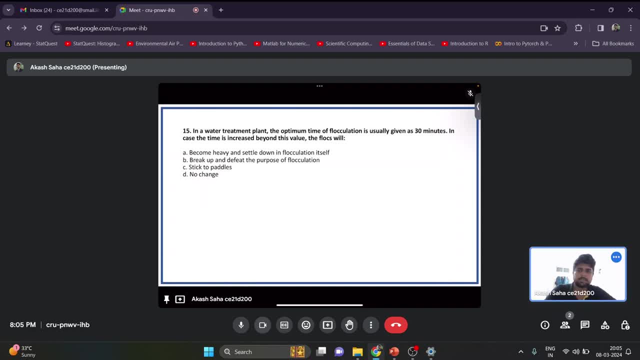 In case the time is increased beyond this value, the flocs will become heavy and settle down in flocculation itself, break up and defeat the purpose of flocculation, stick to paddles and there will be no change. So what will be true in the case if we increase the optimum time of flocculation more than? 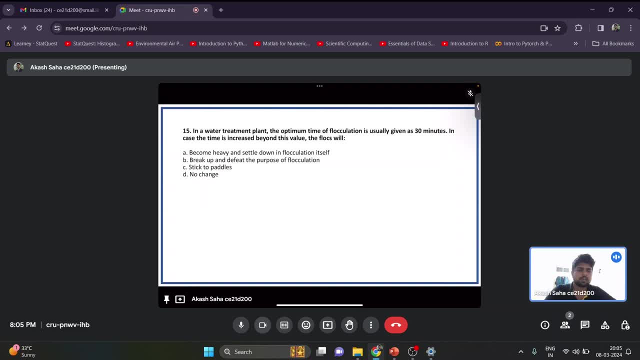 30 minutes. Just think over it, Go through the question. Thank you, There is a question again. So will they become heavy and settle down in flocculation itself? Will they break up and defeat the purpose of flocculation? Will they stick to paddles or there will be no change? So obviously the answer will be: they will break up and defeat the purpose of the flocculation. because more time is given There can be a change case of charge, reversal also, So that can also cause the change. So mostly, if more and more time is given there can be breaking up of the particles. 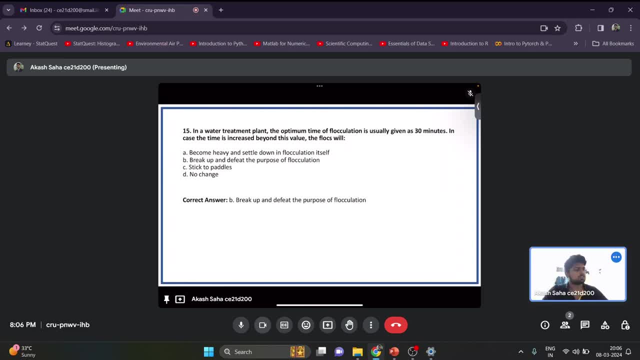 and it will deceive the whole purpose of the formulation. sorption B is characterised case. Again a small numerical: a certain water needs 12 ppm alum, dosing the amount of alum needed for 10 mld of water in quintals per day, or rather, since the options are given, in kgs. 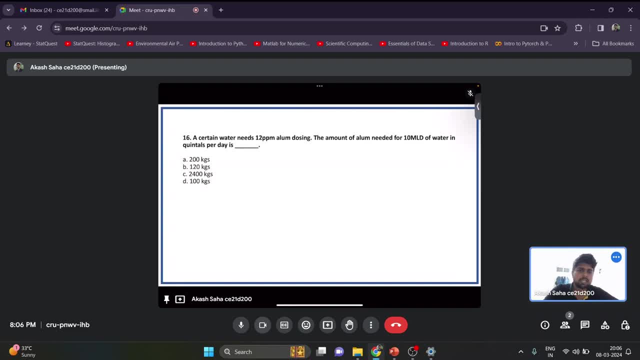 so let it be so the amount of alum needed for 10 mld of water in kgs per day. so rather than quintals, let it be kgs per day, to find out the answer. The concentration is given as 12 ppm of alum and the discharge is 10 mld. so we have to. 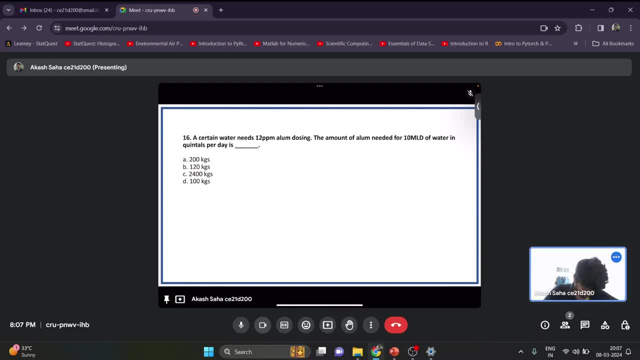 find out the total alum requirement, So we will see the answer. so it will be 120 kgs. so how we will get. So we have the alum dose as 12 ppm, so it is equal to 12 milligram per litre. ppm means 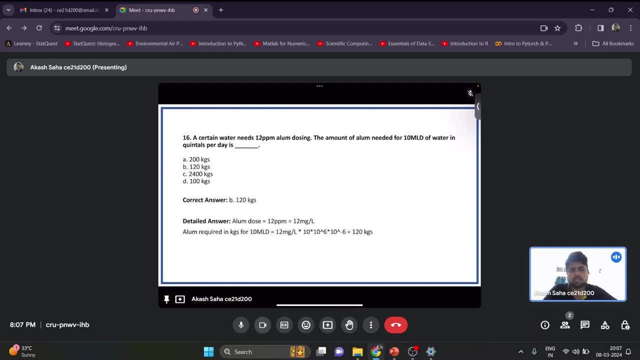 milligram per litre. so now if we multiply it with the discharge, so 12 milligram per litre, into 10 mld, so 10 mld. we can write it as 10 into 10 to the power 6 litres per day. and then to convert milligram into kgs we have multiplied with 10 to the power minus. 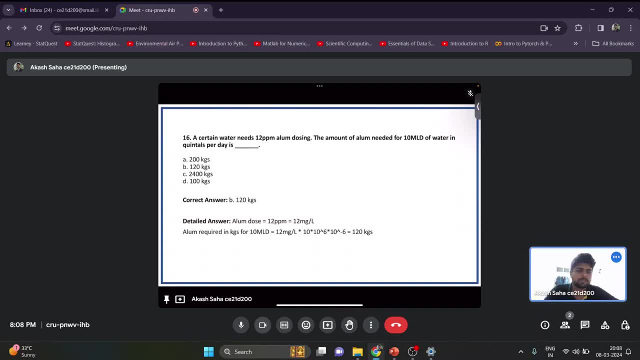 6. So ultimately it will become 12 into 10. So it is 120 kgs. it is pretty simple direct calculation. we will move to the next problem. Okay, select the correct statements regarding turbidity. A. turbidity increase the disinfection. 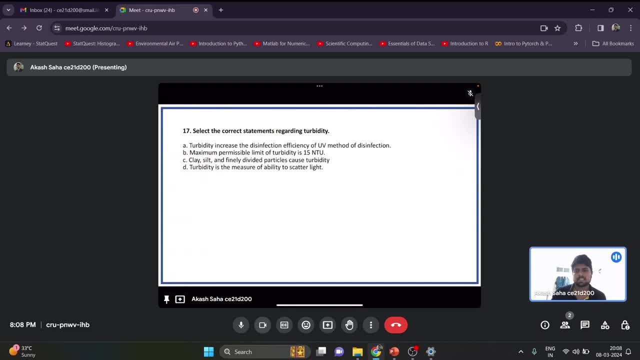 efficiency of UV. method of disinfection. maximum permissible limit of turbidity is 15 NTU. clay, silt and finely divided particles causes turbidity. turbidity is a measure of ability to scatter light. Okay, so just go through the statements one again and we will discuss the correct answers. 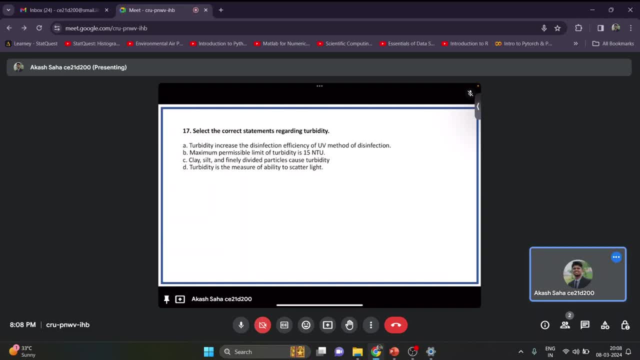 Okay, so let us go through the statements one again and we will discuss the correct answers. Okay, As we see the answer that the turbidity increase the disinfection efficiency. so this statement is false because, due to turbidity, the disinfection efficiency will be decreased. okay, and the 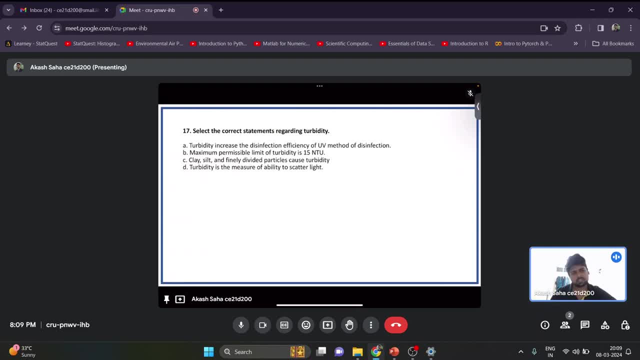 maximum permissible limit for turbidity is 15 NTU. again, it is false. it is 1 NTU, or maximum relaxation up to 5 NTU in case of there is no alternate sources. Okay, Option C: clay, silt and finely divided particles causes turbidity. this is true because all 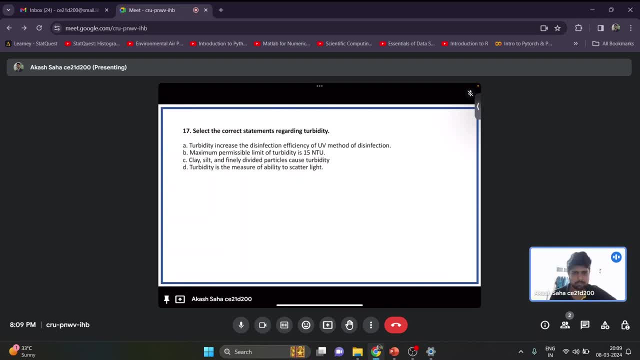 these particles will scatter the light, and turbidity is the measure of probability to scatter light. So again, option D is correct. so option both C and D are correct in this question. so here it is. the correct answer is option C and D. Now we will move to the next problem. 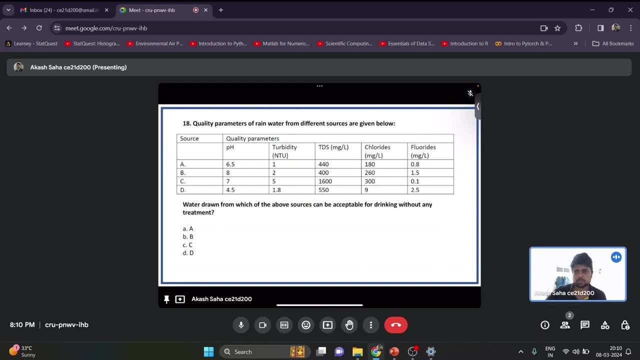 The quality parameters of the rainwater from different sources are given below. so we have the source A, B, C and D where the quality parameters as per pH, turbidity, TDS, chlorides and fluorides are given. So water drawn from each of the above sources can be acceptable for drinking without any. 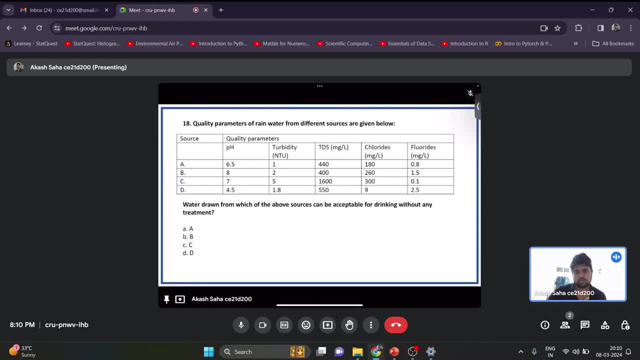 treatment. So we do not want to do any treatment. so we have to check which of the source is correct, is acceptable for drinking without any treatment. Okay, So we are just have to know the drinking water standards. Okay, So we will see these water quality parameters that are, pH, turbidity, the TDS and fluorides. 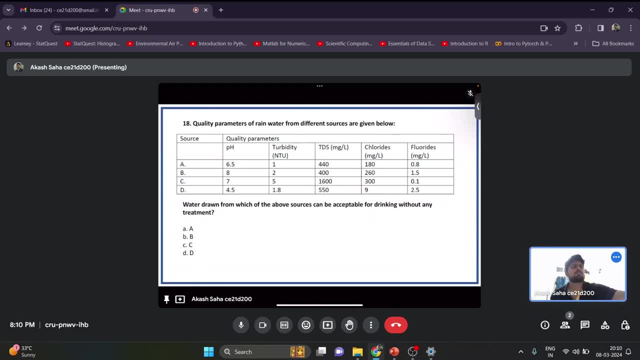 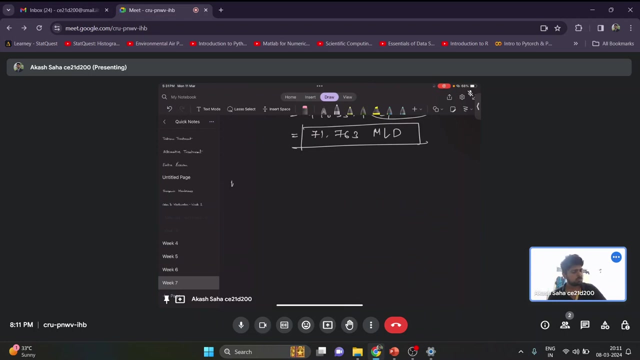 and fluoride, Okay. So, if you see So, we have the Okay Okay, So the Okay Okay Okay. water quality parameters, We have the acceptable limits and we have the relaxed limit, also based on if any alternate sources are available or not. 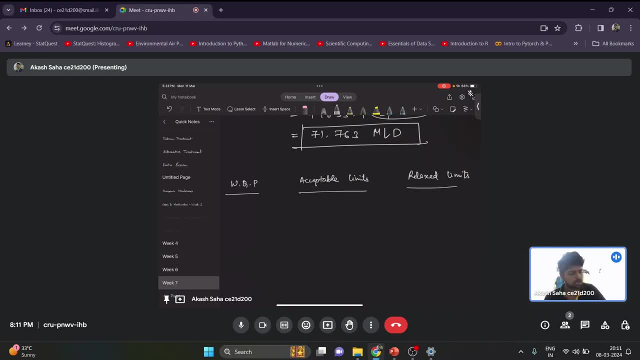 So we will check. So my first water quality parameter is pH. So the acceptable limit is 6.5 to 8.5.. So this is all with respect to is 150500.. So pH should be and there is no relaxed. 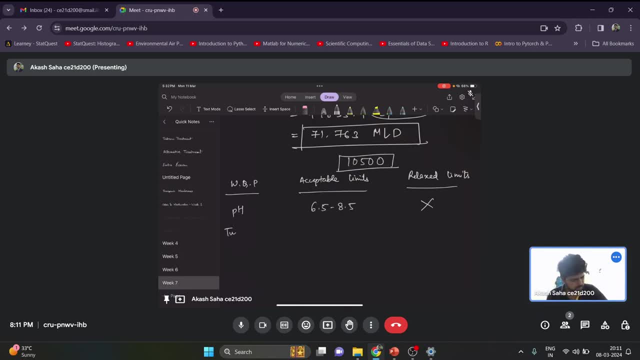 limit, Whereas in the case of turbidity we have 1 NPU and relaxed limit is 5 NPU. In the case of TDS, it is 500 milligram per liter and 2000 milligram per liter In the case of. in the case of chloride, it is 250 milligram per liter and 1000 milligram. 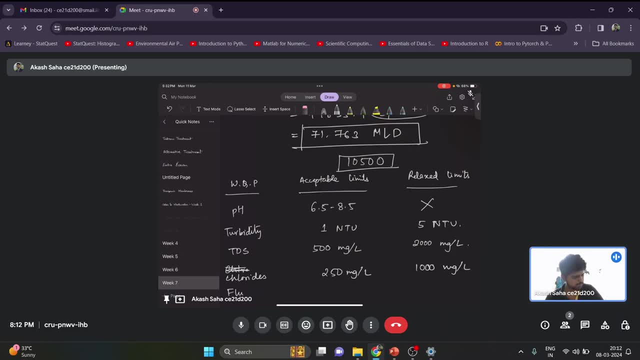 per liter, Whereas in the case of fluorides it is 1 milligram per liter and 1.5 milligram per liter. So we have to see each of the sources and whether they are falling in between These acceptable limits. whichever is, whichever source is falling, that will be the correct. 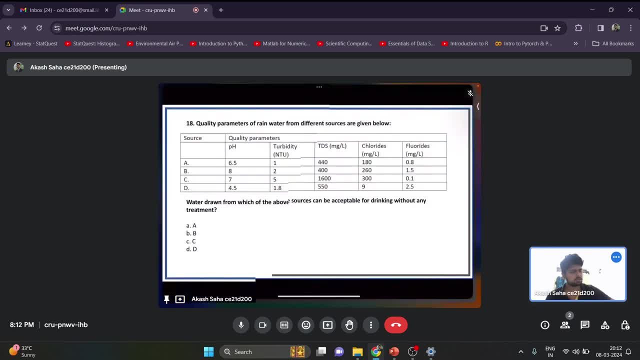 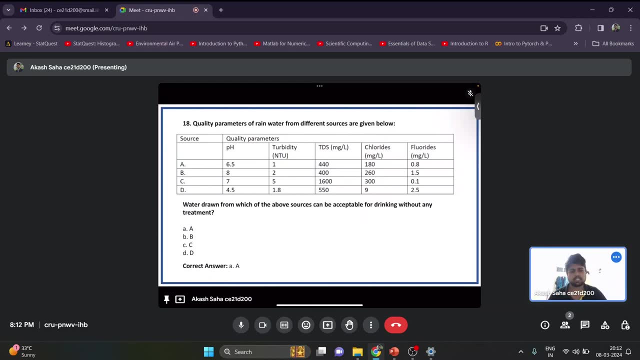 answer. So if we see option A seems to be the right answer because it is falling, it is falling all the acceptable limits of the water quality parameter, so option A is correct. right, We will move to the next question. A: 40 mLd of water is being treated with 18 milligram per liter of alum in a water-treating. plant. Calculate the yearly alum requirement. If the water contains 5 milligram per liter as CaCO3 of alkalinity, calculate the amount of CaO purity of 85% required. So in a particular wastewater in a particular water treatment plant, 18 milligram per liter. 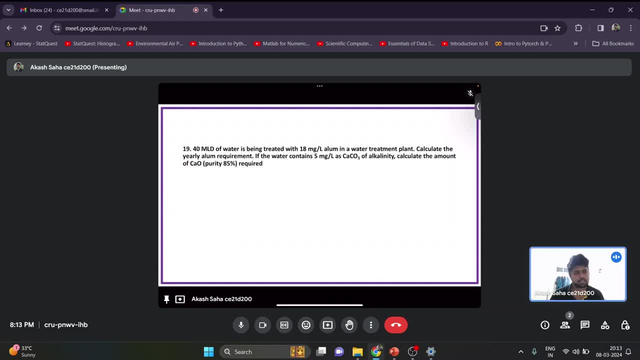 of alum is required. Okay, So we have required for the treatment with a discharge of 40 mLd. So we have to calculate the alum requirement in an yearly basis And also we know that this alum will take up some alkalinity. 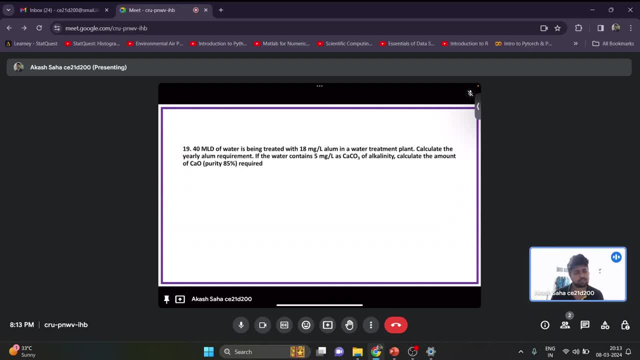 So now the water contains 5 milligram per liter of alkalinity as CaCO3. So how much more CaO has to be provided if the purity is 85%? So this is the problem. Make a measurement, Make a note of it and prior to solve. then we will discuss next further. 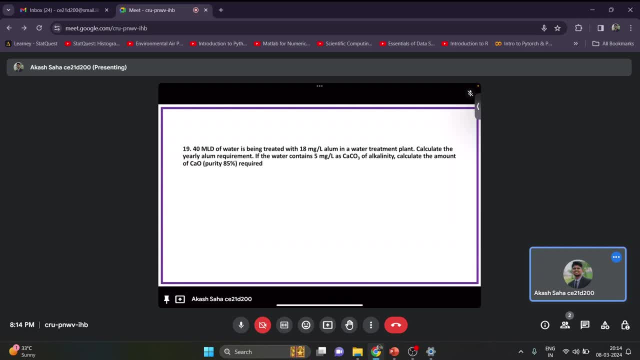 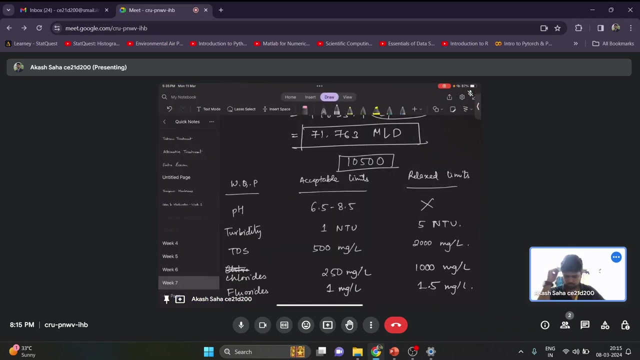 Okay, So we will see how to solve this problem. So this is the problem. so we have this reactor where we are adding 18 milligram per liter of alum and the q that is coming in is 40 mld, and inside this we have already 5 milligram per liter of alkalinity, as 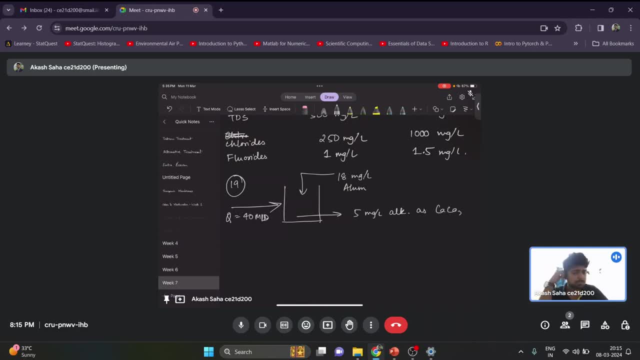 cso3. so mostly alkalinity is given in terms of cso3. that is what is given. so the first part, the yearly alum requirement. so quantity of alum required, it is 18 milligram per liter into 40, into 10, to the power, 6 liters per day. 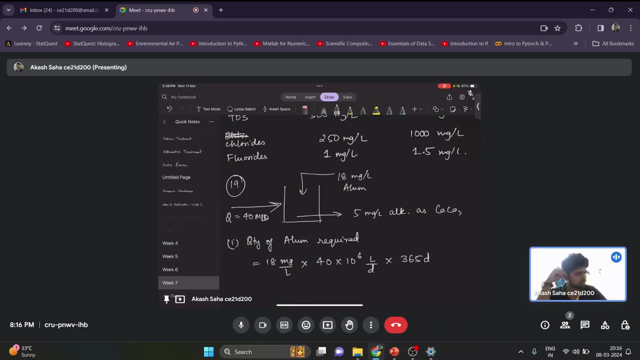 into 365 days and will convert into, in terms of tons, 10 per milligram. okay, so we get it as 262.8 tons per year. okay, so this is the yearly alum requirement. now we have to find out how much cao is required. okay, so this is a thumb rule and we know that one gram of 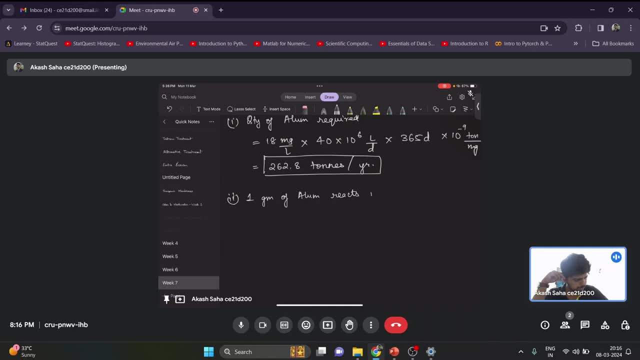 alum reacts with 0.45 grams alkalinity as cao3. so by the chemical formula and reaction we know that one gram of alum will react with 0.45 grams of alkalinity as cao3. so now here we have 18 milligram per liter of alum. 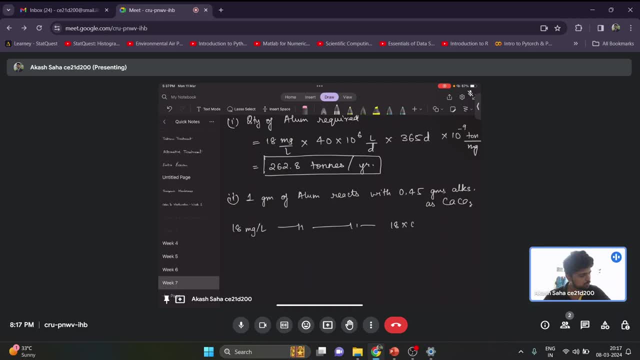 and this will react with 18 into 0.45, which is equal to 8.1 milligram per liter alkalinity as tsa3. okay, so the additional additional alkalinity go required will be 8.1, And 5 is already there in the system. so 8.1 Minus 5, so 3.1 milligrams per liter. okay, so 3.1. 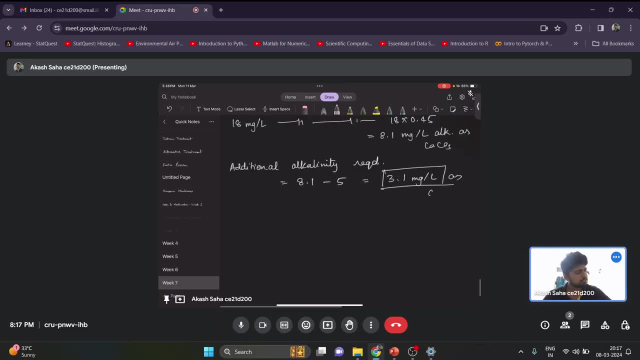 milligrams per liter, as cso3 is, as cao3 is required. okay, so now we are doing with respect to the calcium oxide, cao. so we know that cao will react with alkalinity, give probability as CaOH twice. So we will correspond this to 1 CaCl3.. So this is one. 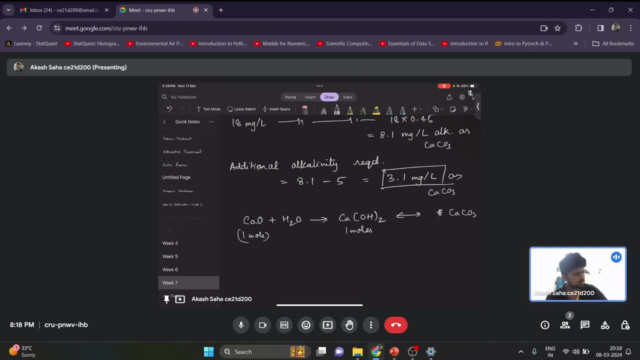 mole. we will give one mole of this. we will give one mole of this. So we can say that one mole, CaCl3, is induced by one mole of 100 % CaO. So one mole of CaCl3 is induced by. 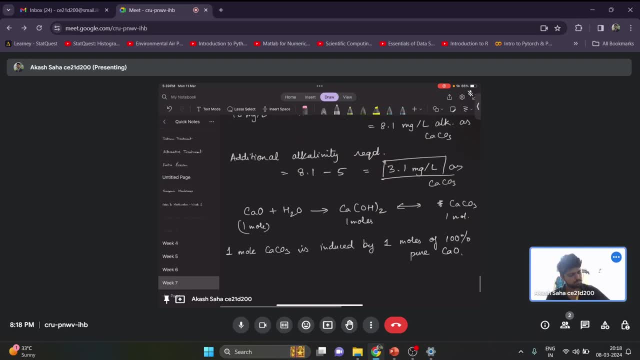 one mole of 100 % CaO. or we can also write one mole of CaCl3.. I am trying to think to 100 grams. 100 grams CaCO3 is induced by 1 mole of CaO is 56 grams. 56 gram of CaO. 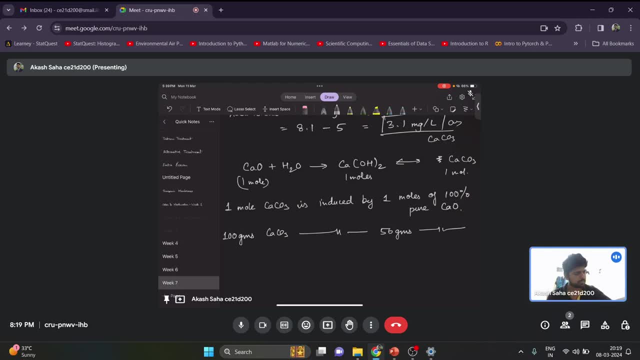 So we need 3.1 milligram per liter as CaCO3.. So 3.1 milligram per liter as CaCO3 is induced by how much It will be equal to 56 by 100 into 3.1 milligram per liter. 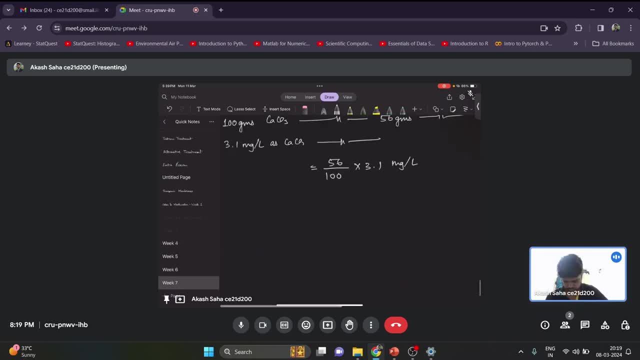 Just in statements we can find out the answer. So the quantity of 85 percent CaO, CaO, that will be equal to how much 56 by 100 into 3.1 milligram per liter. Now it is 85 percent CaO. 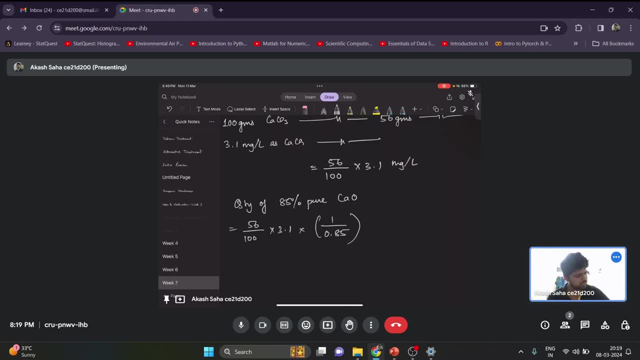 So 1 by 0.85 into the discharge, 40 into 10 to the power 6 and into 365 days, and to convert into tons we will get 10 to the power minus 5.. So this is the overall quantity We will get it. 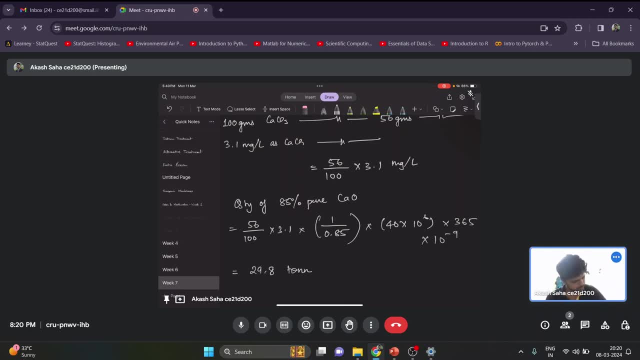 as 29.8 times 5.. So I think it is pretty simple. So 29.8 times per year of Ca is required to do the coagulation, So we can go through it once again. So first we will calculate the alum requirement Directly. 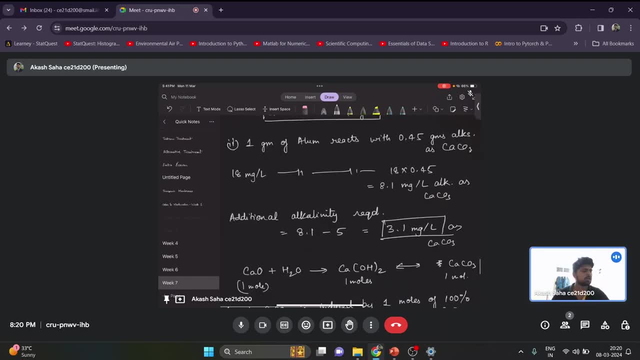 we will multiply it with the discharge. Then we know that 1 gram of alum reacts with 0.45 grams of alkalinity as CaCO3.. So 18 milligram per liter. that would be 8.1. So now 5 is already present in the system. So 8.1 minus 5,. 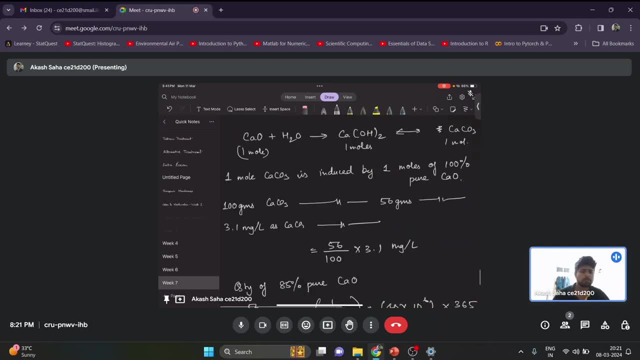 additionally, 3.1 is required. So now 1 mole of CaCO3 is induced by 1 mole of CaCO, or we can write it as: 100 grams of CaCO3 is induced by 56 grams of CaCO. because of that molecular weight, 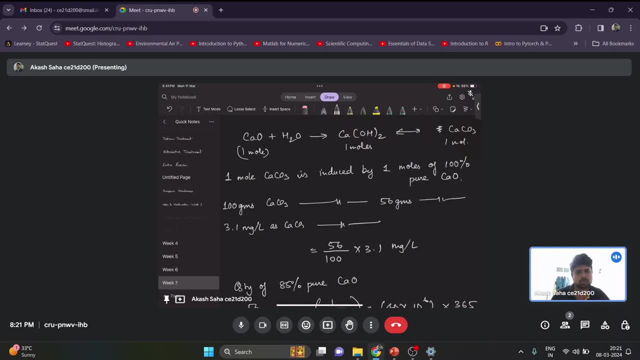 So 3.1 will be induced by 56, by 100 into 3.1.. So for 85 percent Ca you have to just divide, divide by 0.85 into the discharge, into the number of days, 365 into the unit conversion.